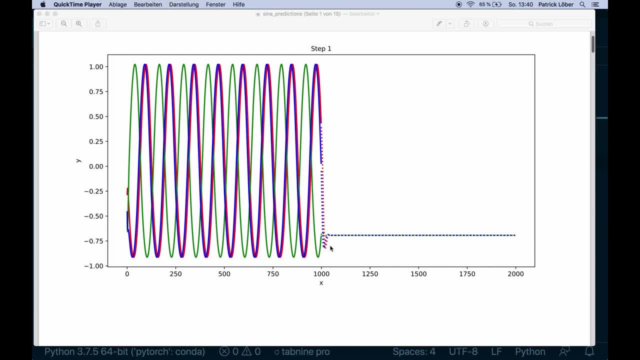 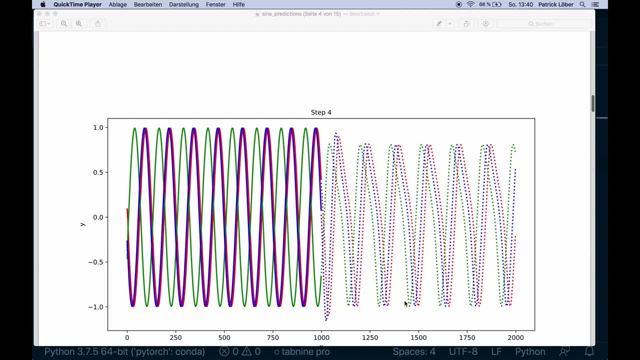 we can see that our network is not good at all. So these are our predictions. But then with each training step it will get better and better and predict the sine wave in the future. So this is a relatively simple example, But the concepts we use here can be applied to. 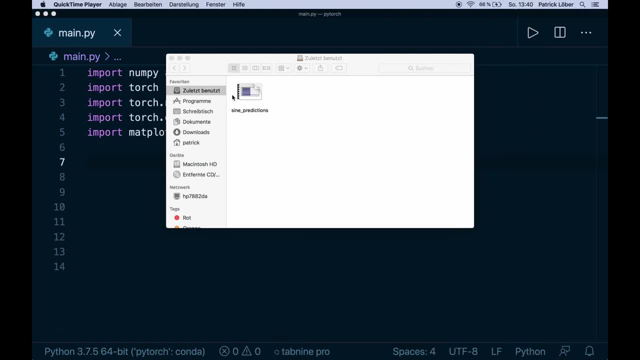 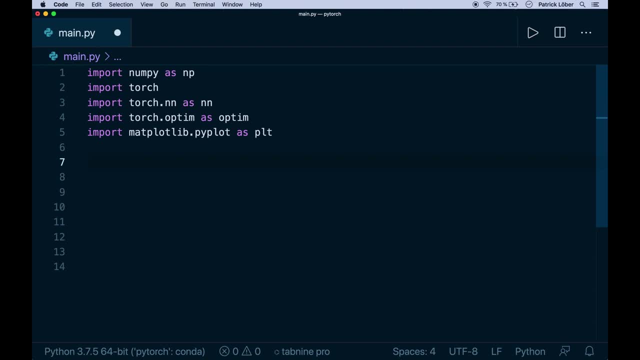 any time series prediction. So let's jump to the code. And here I already have all the imports we need. So the first thing we want to do is create our data. So we want to create values for a sine wave, So let's create some parameters for this. So let's 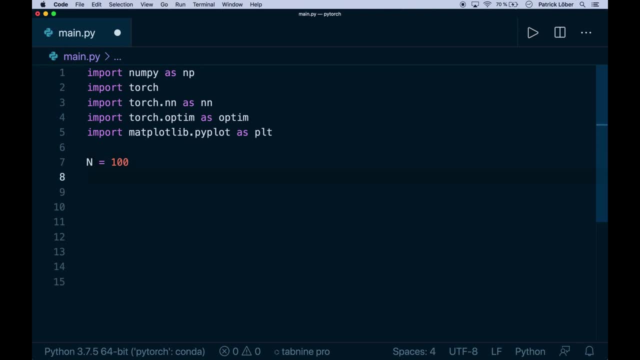 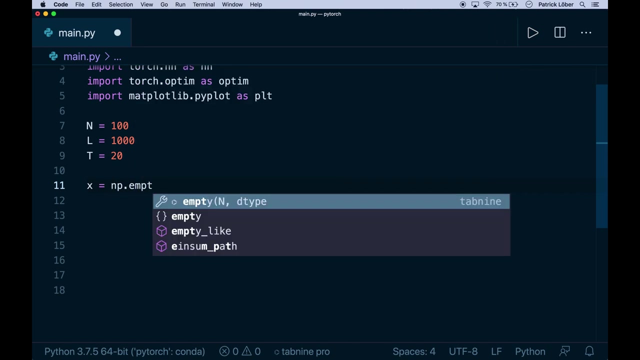 say the number of samples should be 100.. L is the length for each sample, So the number of values we have for each sine wave. And then we also have a parameter t that specify the width of our wave. So let's create some samples. So we say x is a NumPy array And this should be a empty NumPy array. 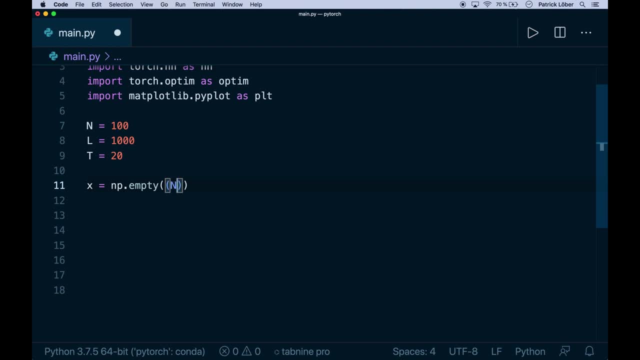 And as shape we give it the size n and L. So m again is the number of samples and L is the length for each sample. And we also give it a data type, So we say float 32.. Then we want to shift. 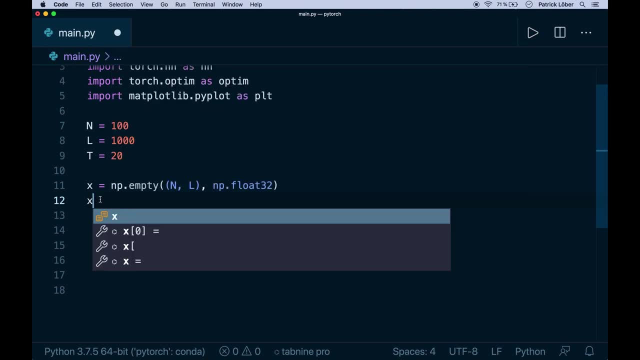 each sample little bit randomly. So we say x and then colon, So for each, for each sample, and then all values. we want to shift this a little bit. So we say the values are a numpy array in the range of L, So this will give us values between zero and 999.. But now we want to shift. 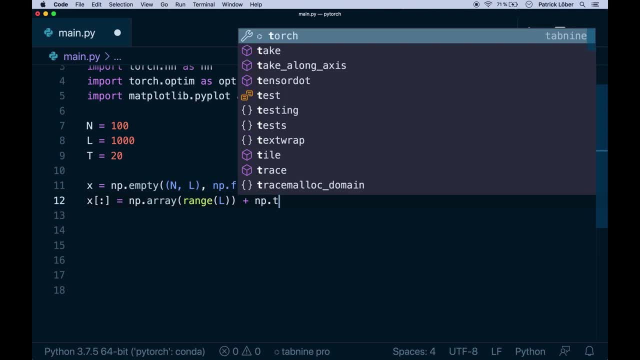 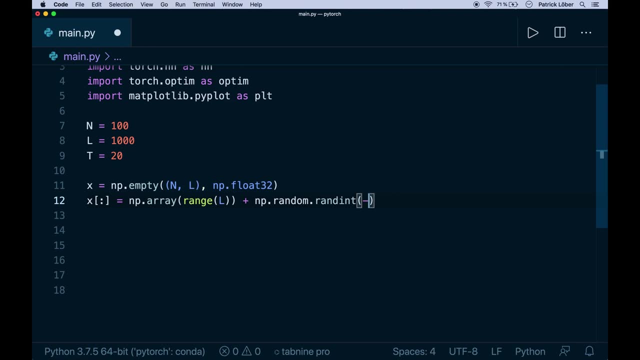 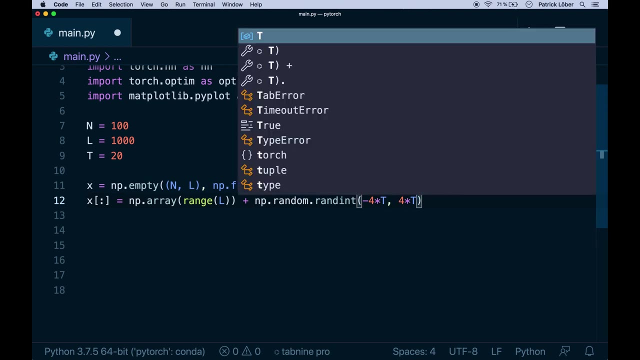 them a little bit. So we say plus numpy, and then we say random, and then random int, And now the range should be from minus four times T until plus times for times t, and then we need to give it the shape. So this should be n, and now we have to reshape this. 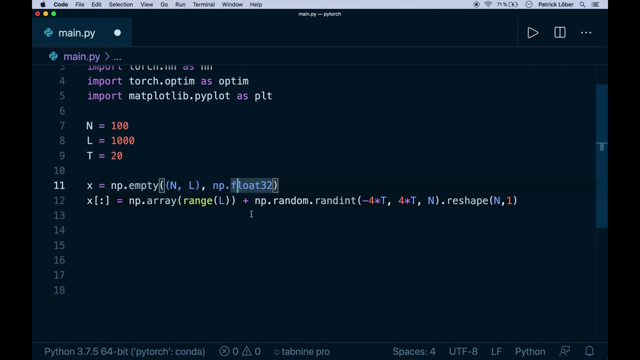 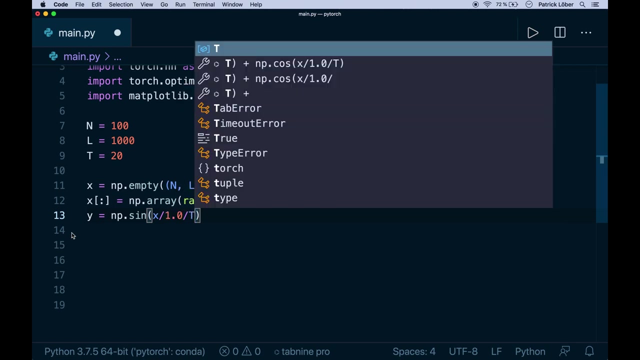 So it must be in n and one, Otherwise we can't apply the plus here. So now we have have this, and now we want to create the corresponding sign value. So we say y equals numpy dot sin. And now here we say x divided by 1.0, divided by t. So this will just specify the width. 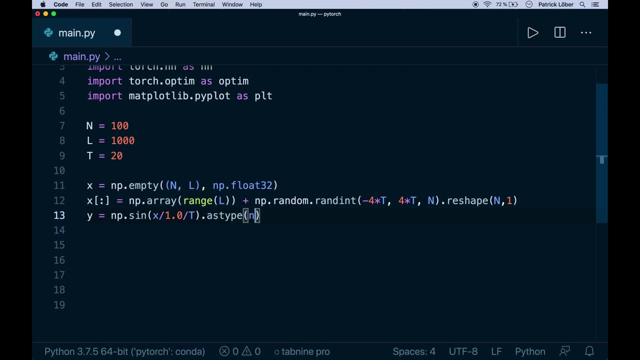 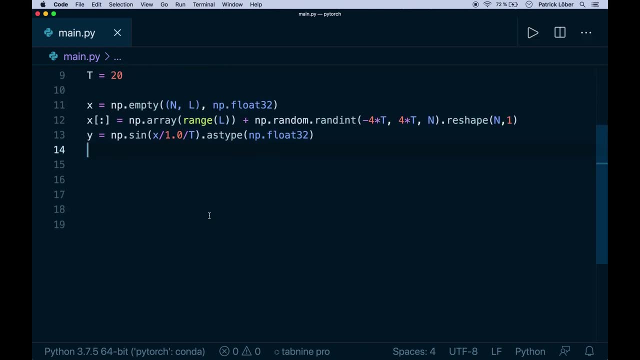 And then we want to have this s type, And again here we say: numpy, float 32.. And now we have this. So let's actually plot this so that we can see how this looks like. So for this we create a numpy, a sorry, a matplotlib figure, And this should be our. here we can. 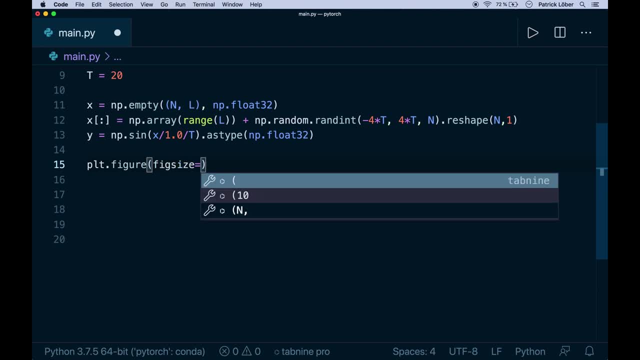 give it a fixed size, And this should be, let's say, 10, and then eight. And then let's give it a title- PLT dot title- And let's say this should be a sign wave. Then let's also define some x and y labels. So PLT dot, x label, And here we just say x. 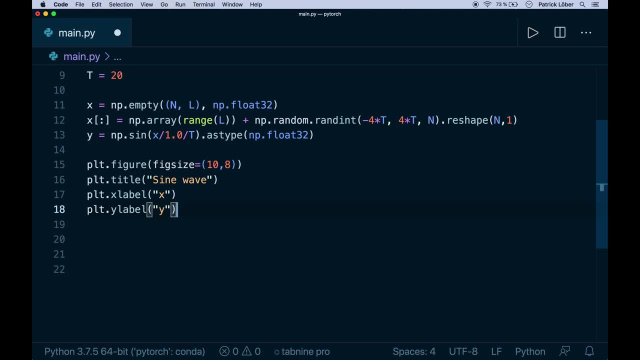 PLT dot y label. we say y, then we also want to have x and y tech ticks. So we say x ticks and give it a font size of, let's say, 20 here and the same for the y ticks. So y ticks, sorry, y ticks. 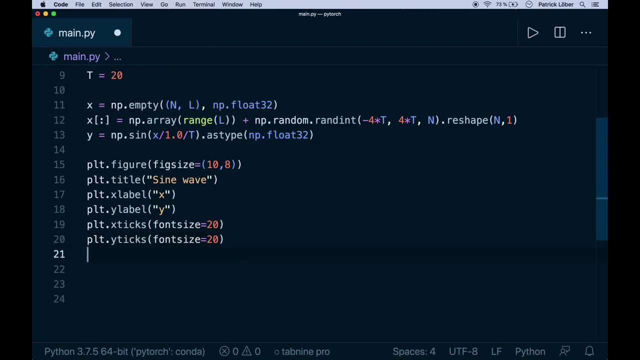 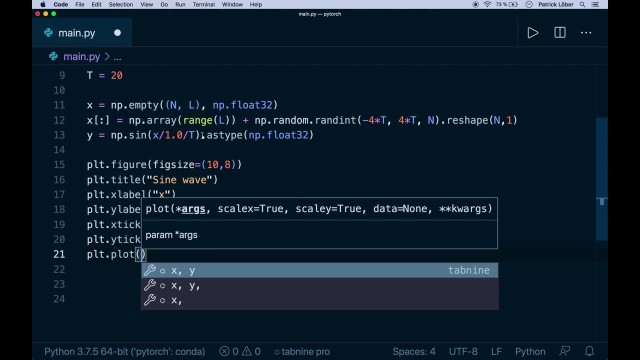 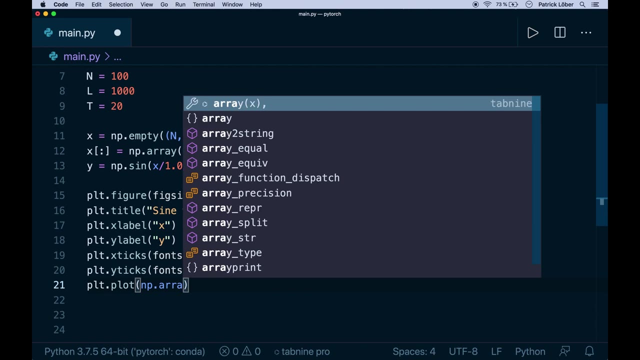 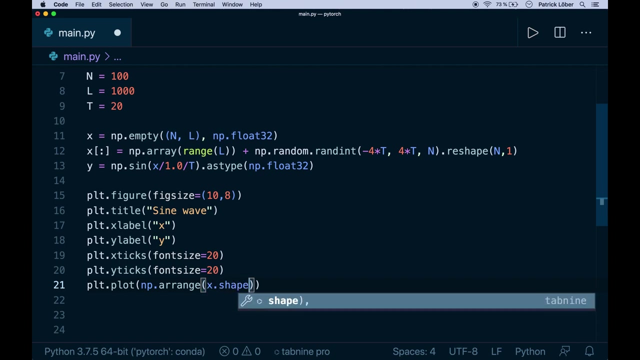 And here again the font size should be 20.. And then we want to plot the actual points. So here we want to plot points from zero to 999.. So we can get them by saying numpy a range. then here we have to say x, dot, shape, and then the first dimension. So this will be. 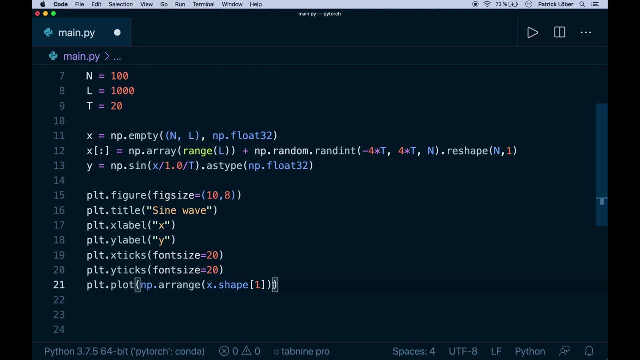 1000.. And as the second parameter that we want to plot. so here we want to plot y And here we want to plot only one sample. So we say the first one, zero, and then all the values, then let's give it a color red And let's also give it a line width of 2.0.. 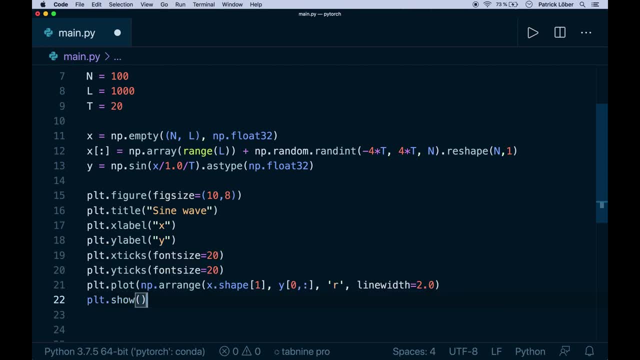 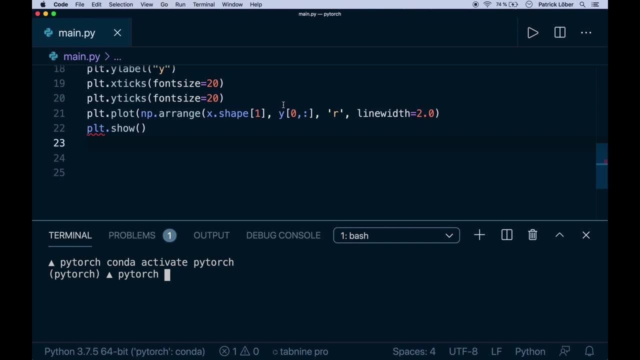 And then we say PLT dot show. So now we have our sine wave. So let's actually run this and see if this is working. And here I see I have a parentheses missing. So let's say Python, main dot pi. And I also have a typo here. 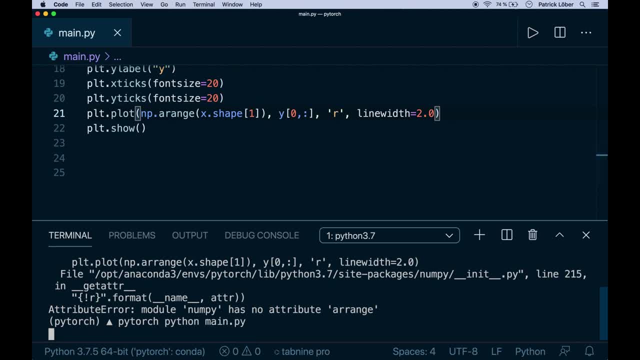 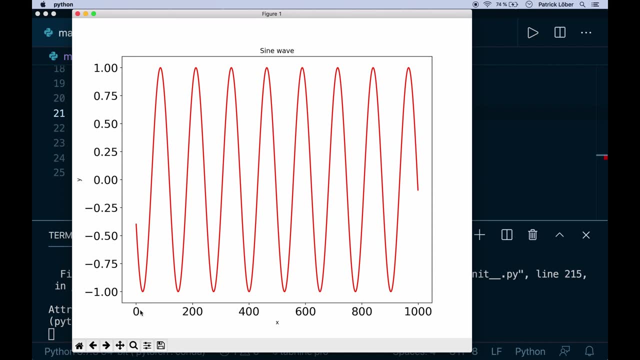 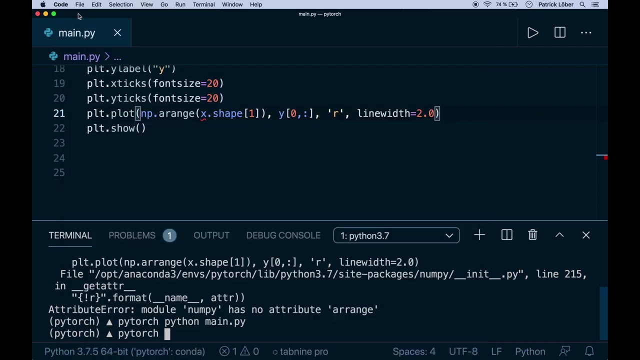 With a numpy, a range with only one R. So let's try it again. Alright, so this works. So here we have our sine wave from from zero up to 1000.. And now for the next 1000 values. we want to predict the values. So let's do this, So let's comment this out Again. we 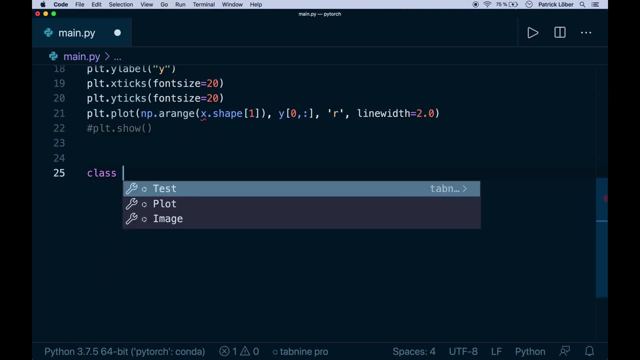 don't want to plot this now And now. let's create a class and we call this LSTM, Let's call this LSTM predictor, And this must inherit from N N dot module. then we first redefine the init method, which gets self, And we also give this a parameter number of hidden. so the hidden. 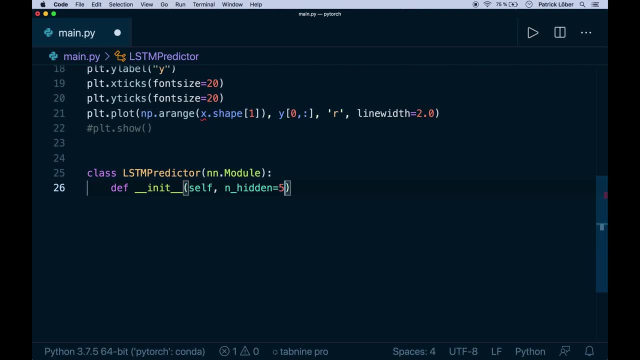 size and let's give it a default value of, let's say, 51 here, So you can play around with this. And now the first thing we want to do is call the super initializer, like so: And then let's say 0.5. And then let's say 0.5. And then let's say 0.5. And then let's. 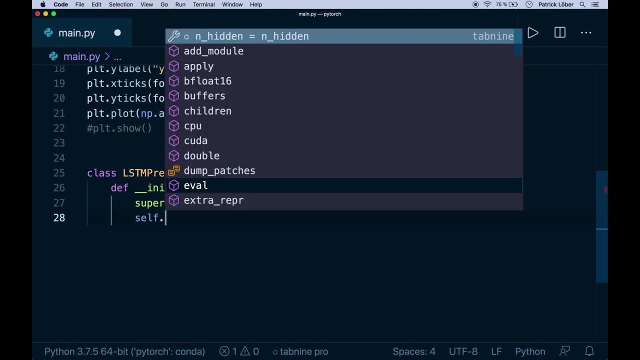 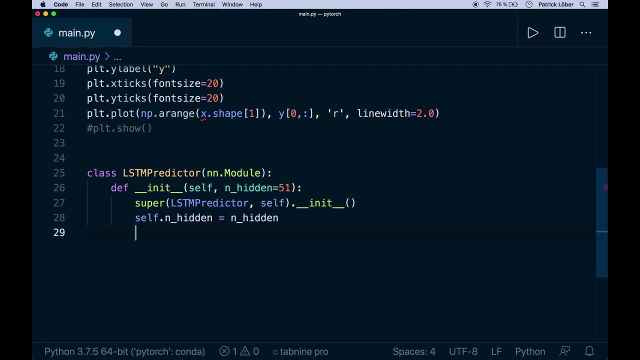 let's store the hidden size. So let's call, So let's say self dot n hidden equals n hidden. And now we want to create our different layers. So in this example we want to apply to LST m cells so LST m one and LST m two, And at the end we want to have a linear layer, because 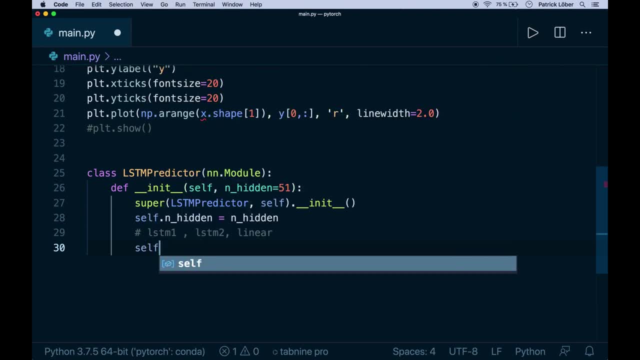 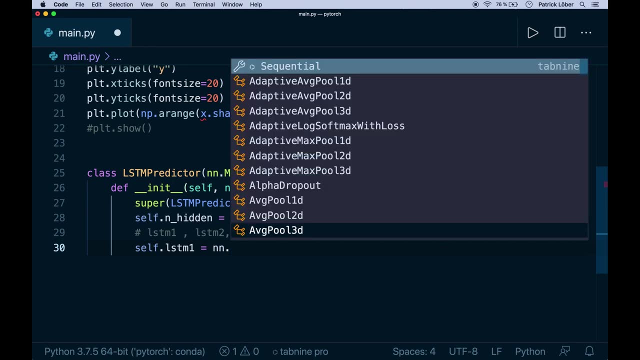 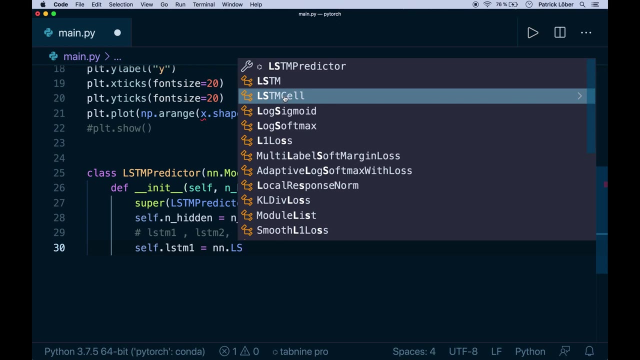 we want to do a prediction, So let's do this. So let's say: self LST m, one equals. and in this case we say n n dot LST m cell. So notice, there is an LST m and an LST m cell. So there's. 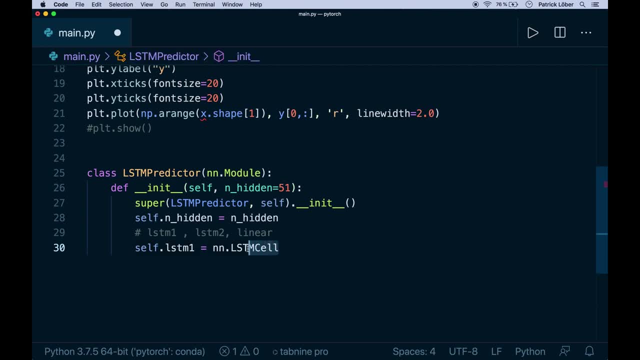 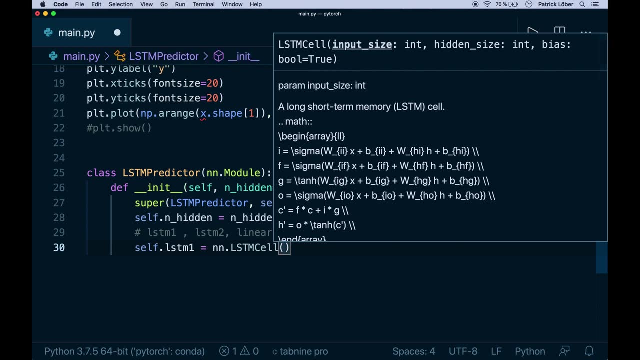 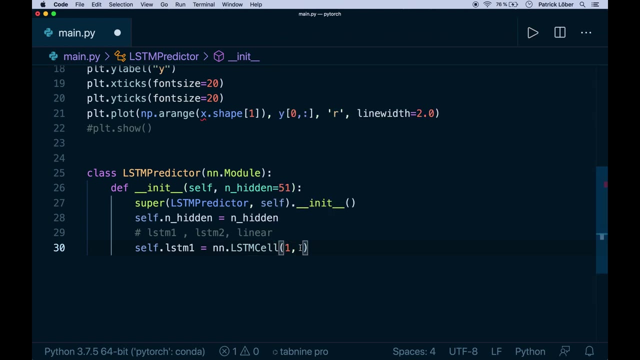 a slight difference and then LST m cell just will give you a little bit more flexibility. So in this case we want to use this one and we have to give it a, a input and a hidden size. So as input we just say one, because we go over our sign values. 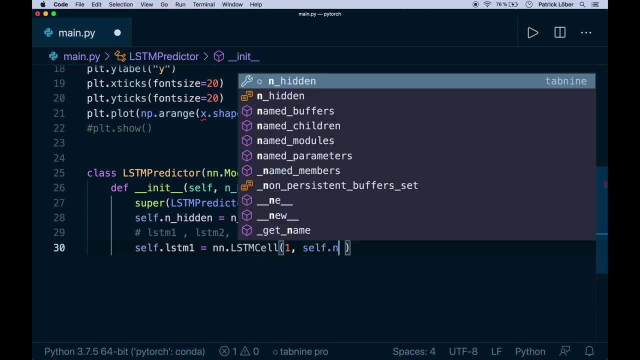 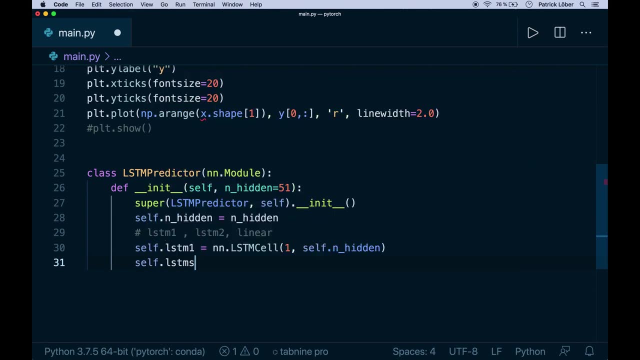 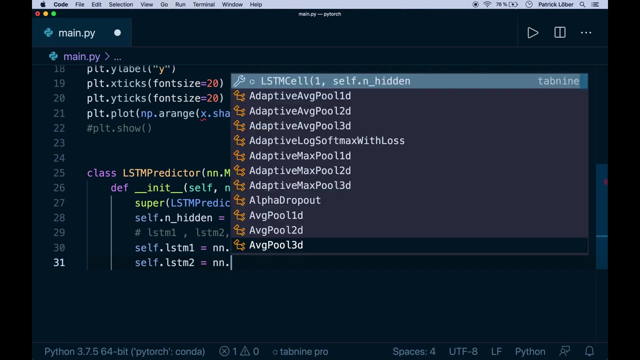 one by one. And then here we say: self dot n hidden. And then we want to stack two LST ms together. So we say, we create another LST m cell and say: self dot LST m, two equals n n dot LST m cell. And now here as the 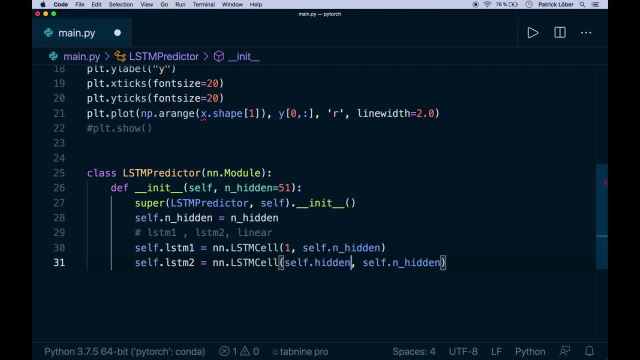 input. we just say one, because we go over our sign values one by one. And then here we say self dot n hidden. And then we create another LST m cell and say self dot n hidden. And then we create a linear layer. So we say self dot linear equals n n dot linear. And now here, as the input size, 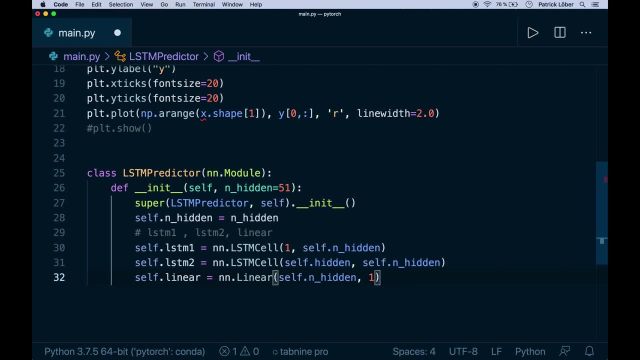 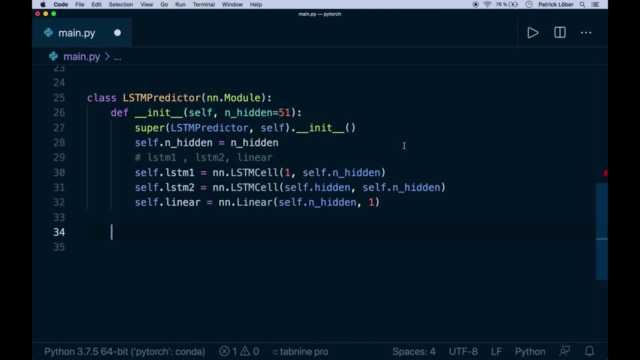 we say self, dot, n hidden, and as the output size one, because we only predict one, it will give it a single value for our sine wave. So this is the y value. Then we define the forward function and this get self and it also gets x and it gets an optional parameter that we call future. 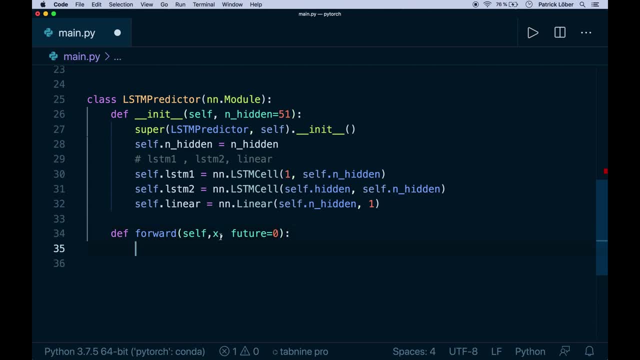 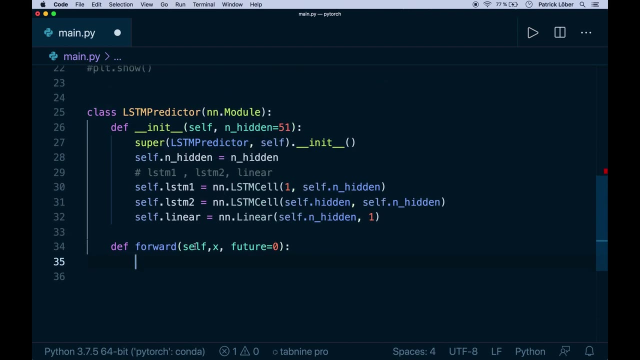 And by default this is none. So if we specify the future value with, for example, 1000,, then this would mean that we also want to predict the next 1000 values, And if we just say zero, then we don't do the future prediction, but only do the training. 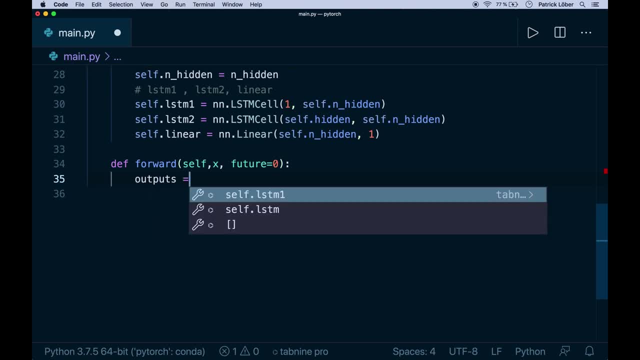 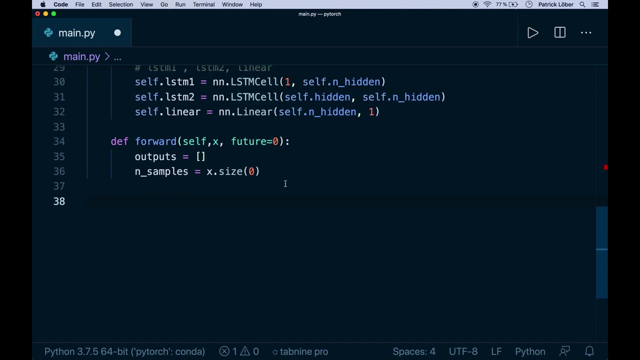 on the values that we know. So here we create an outputs array. So this is just an empty list in the beginning. then we say: the number of samples equals x, dot size: zero. So because we need this multiple times, And then for the LST M cell we need a hidden state and a cell state. So first, 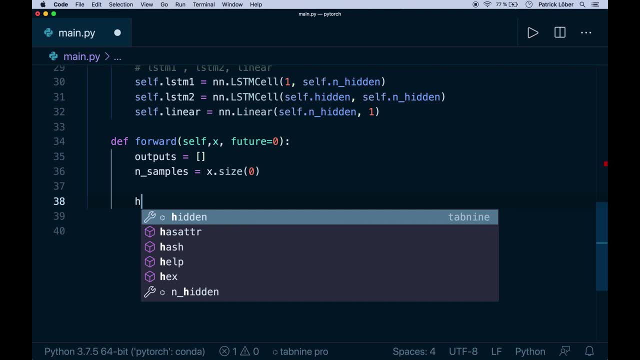 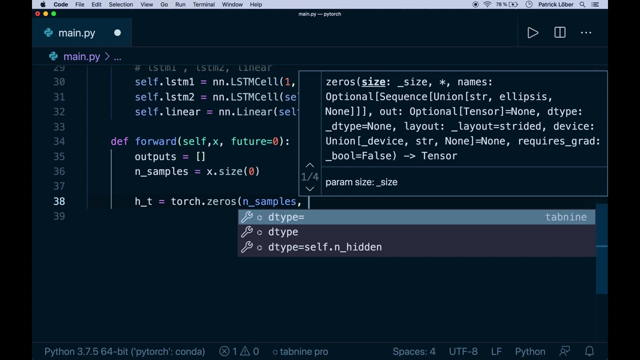 we have to create an initial state with zeros. So we say let's call this HT equals and then torch dot zeros and then as the size. So here we say number of samples and then the next value should be the hidden size, self dot, n, hidden and as data type. 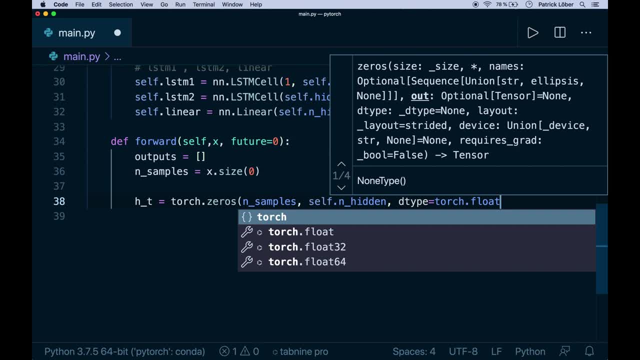 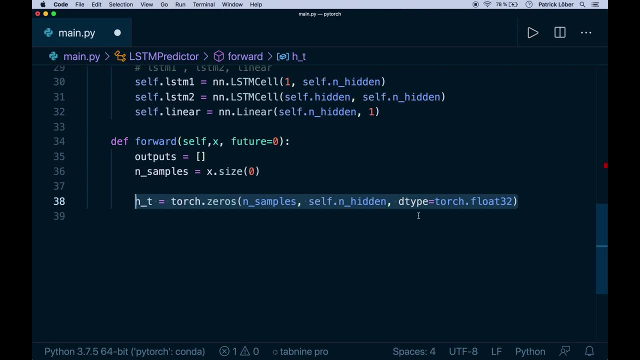 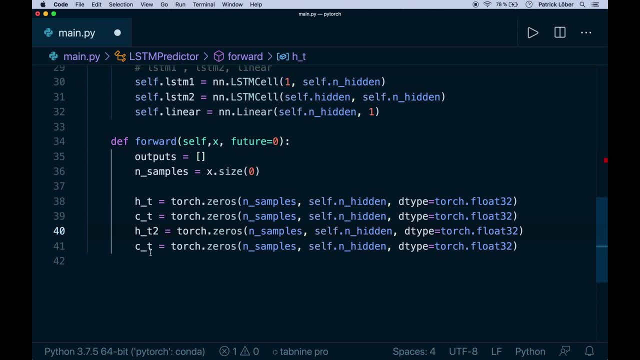 need the very same thing for our second LST M cell. So let's again copy and paste this And let's call this HT two and CT two. And now we want to go over our tensor x one by one. So that's why we 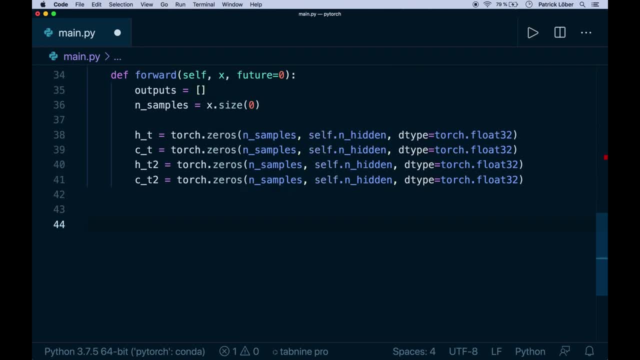 used one as an input here. So for this we could just do a normal for loop and get the current index and then do a slicing operation with our tensors. But there's an even better way with PyTorch. So we can do this directly by saying for input T. 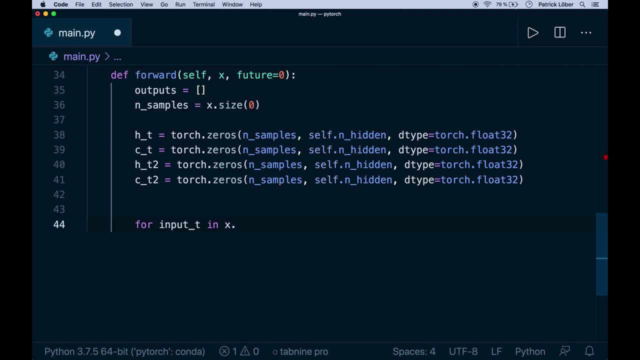 in. and then there's a function that is called x dot split or torch dot split, And here we need to give it the chunk size. So in this case we say one and we want to give it a dimension of one. So this will split the tensor into chunks. 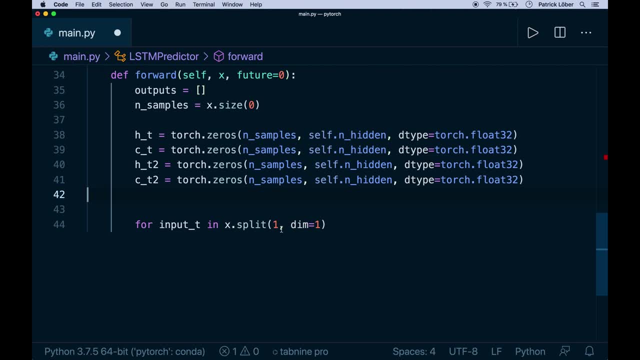 And each chunk is a view of the original tensor. So this just will split our tensor in one value chunks. for example, if our whole tensor, for example, has the size n, so our batch size, and then 100. So then in here we will get n and then by one only. So we do this one by one And 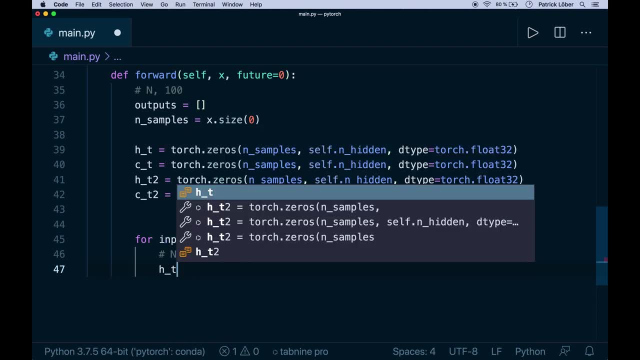 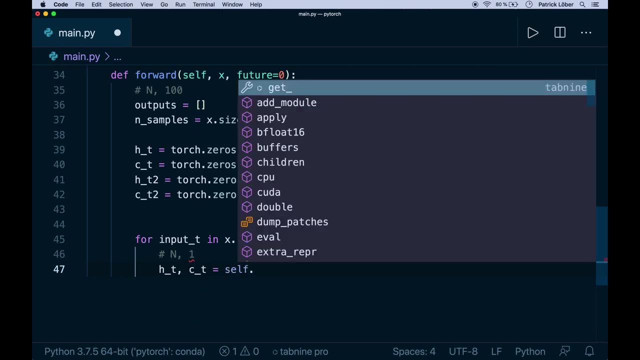 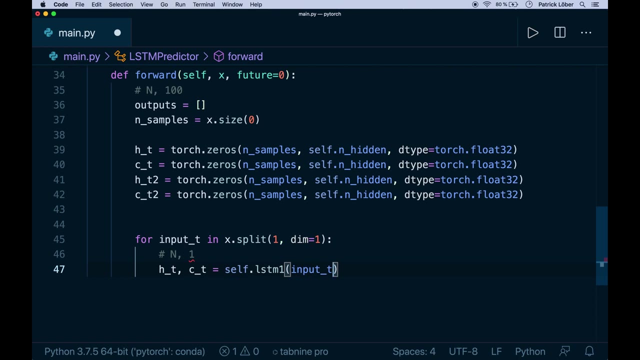 here we call our layers. So first we call the first LST M cell. So we say HT and CT equals self dot LST m one. And now as an input we say input T, And then as a tuple we need the initial hidden state, HT and CT. 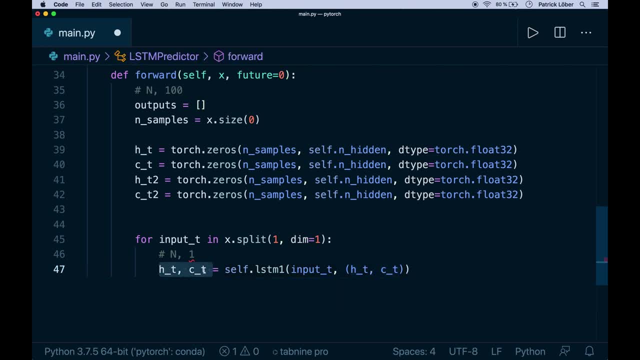 And this will output them again. So we will store them again in those cells And then we call the same for the LST m two, so our second LST m cell. but now the input of this one is actually an input h2.. So this is the hidden state of the previous one, And here we store them in h22 and ct2.. 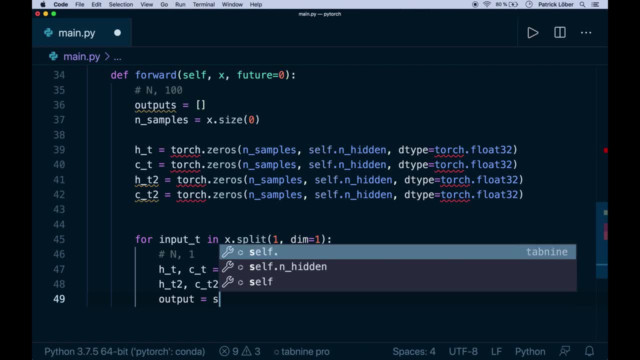 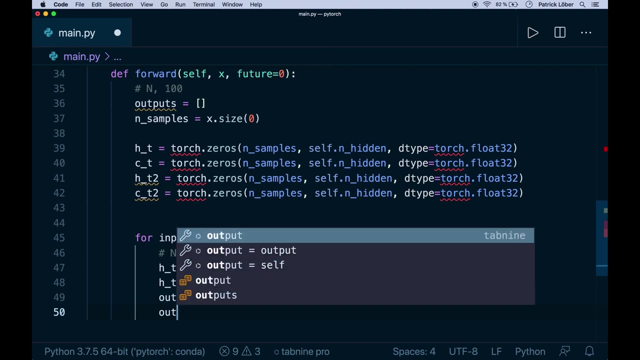 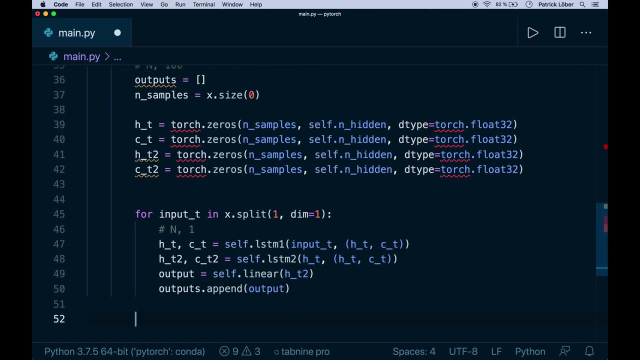 And now our output equals. now we apply our linear layer to get the prediction, So self dot linear of h, t, two, and then we append our output to our outputs array. So we say out puts and then dot append our output, And now we have this. and now, if our future value 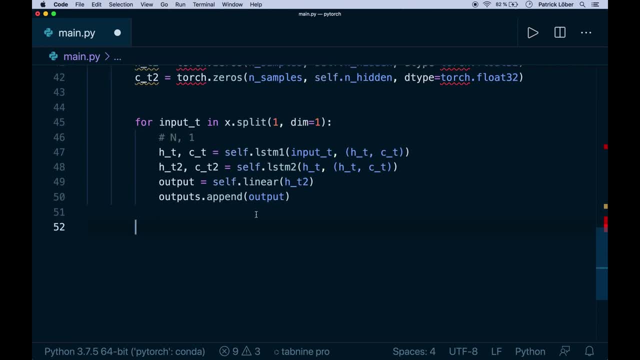 is greater than zero, then we want to do the same thing for the future values. So we say for i in and then range future. So if this is zero, then we won't go over this loop at all And in here we do the. 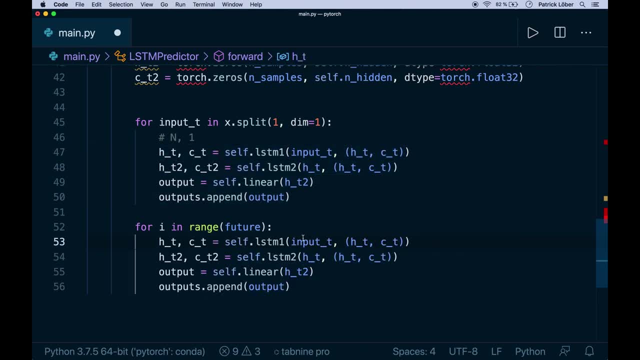 same thing. So here, first we call the first LSTM, then the second one, then our linear one, and then we append it to the outputs. And now, here we have to be careful. So now the input for the first LSTM is the previous output, So this one, so this is used to get. 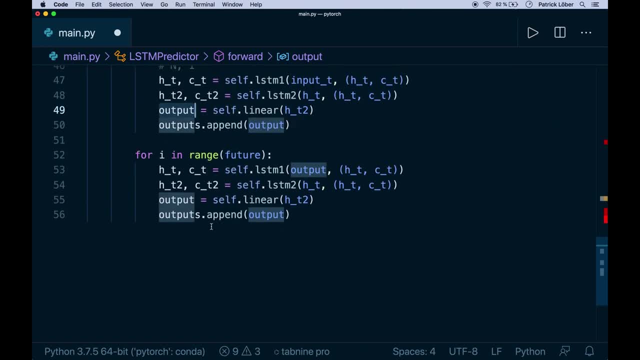 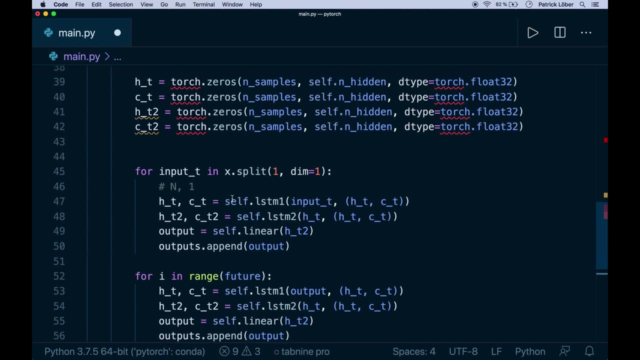 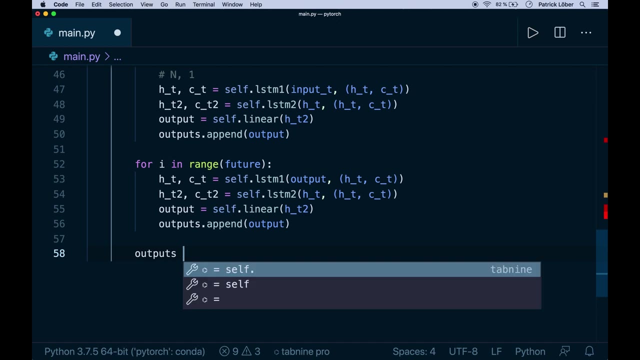 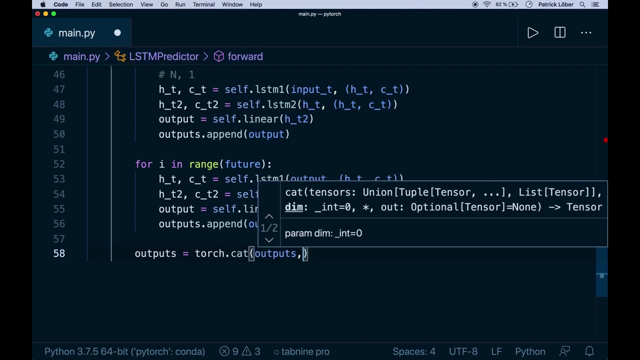 the next output for the future. And now that we have that, we simply want to concatenate our outputs and put it into a torch tensor. So right now this is a list, So here we say outputs equals, and then we can use torch dot cat and use the outputs, and then we also need 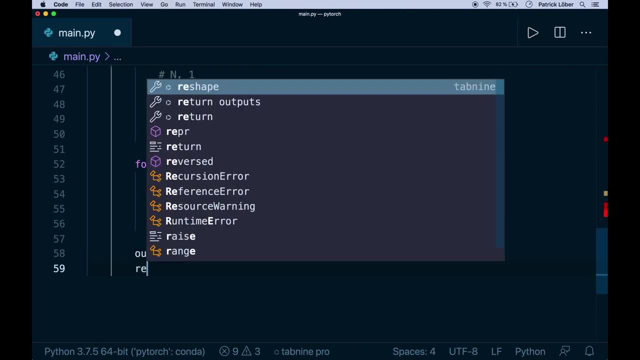 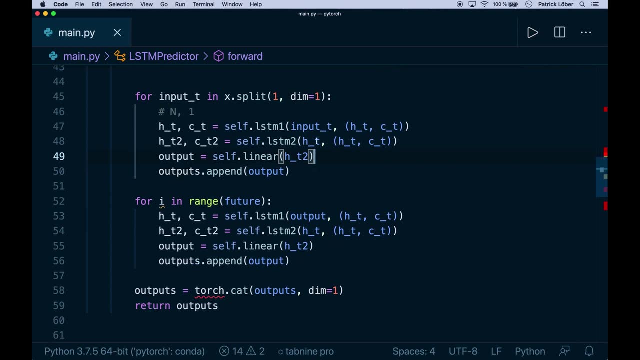 to give it the dimension equals one, And then we return the outputs. Alright, so this is the future me, And here I realized a dump mistake that happened through copy and paste. So here I want to say HT two and CT two for the second. 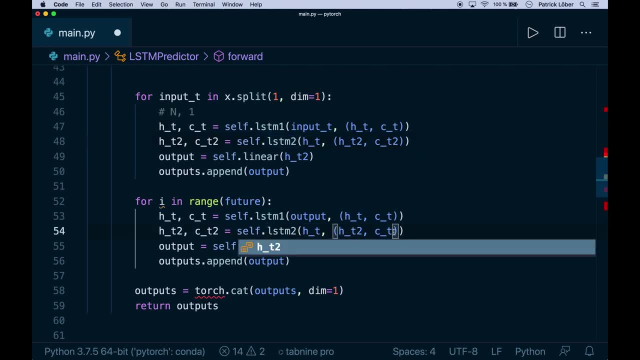 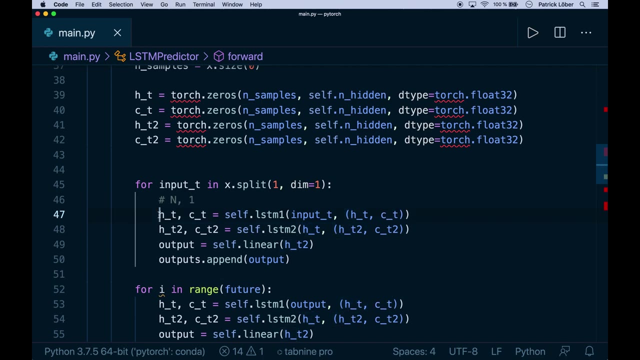 LSTM cell and the same down here, HT two and CT two. So again we call the first LSTM cell with the hidden and the cell states for the first cell, And then we use the output of the first cell as input for the second cell. But here we 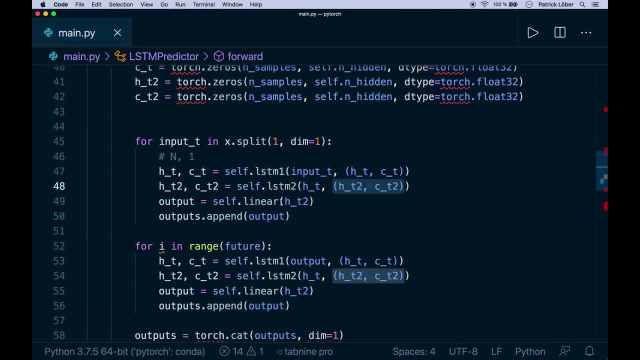 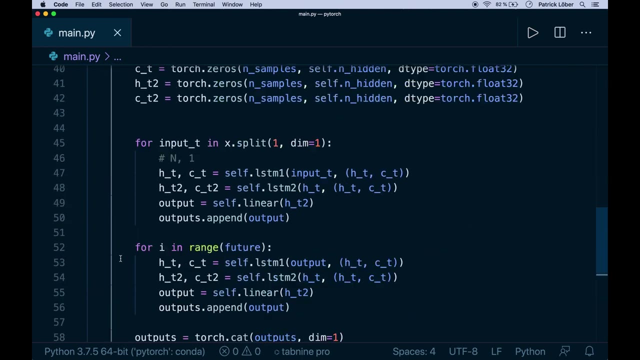 use its own hidden and cell states, And then again we use the output of the second LSTM cell as the input for our linear layer. So now it should be fine, And this is all that we need for our models. So now we have an LSTM predictor that can take an input value. 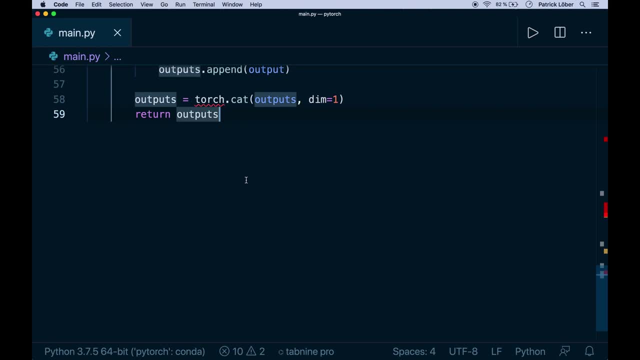 and do Few Future predictions. So now let's actually test this. So for this we say: if name equals, equals main. So now the first thing we want to do is generate some training and testing samples. So let's call this train input. And here we say: this is torch dot from numpy. 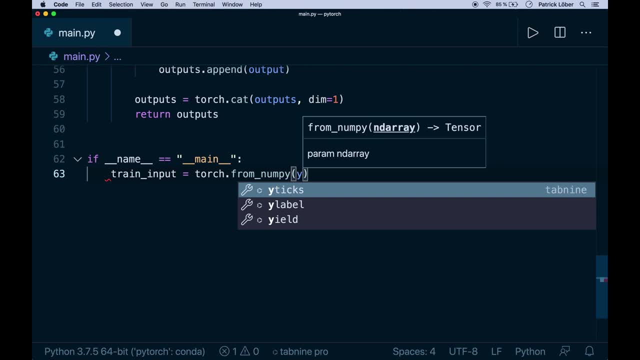 And then here we put, we put in y, And now we start at bed batch three or example three. So we say three colon to the end, And for the values we start at the very beginning and go until the last value, and this is excluded. And now 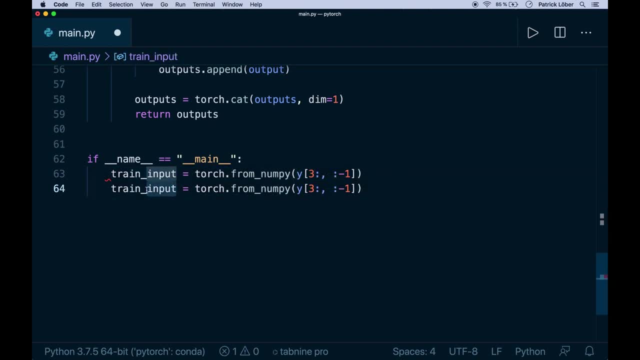 for the training target. So this is the values we want to predict. we do the same thing: we take the samples starting at three, and here we use the value starting at one and go all the way, all the way to the end. 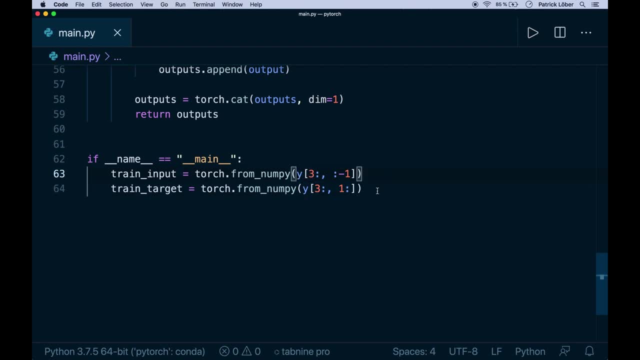 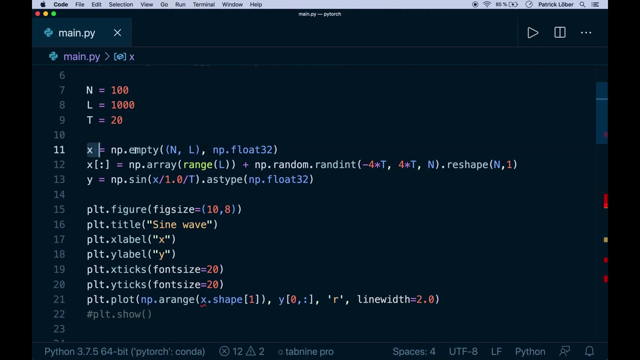 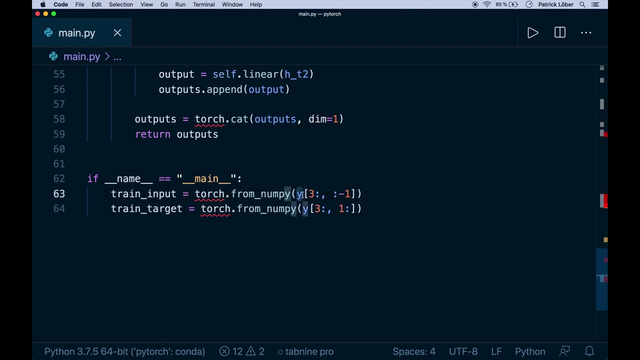 So this is a little bit tricky here. So the first thing you should notice here is that for the input we don't use x, So we don't use this at all. But what we want to do here is we only want to look at the y values. 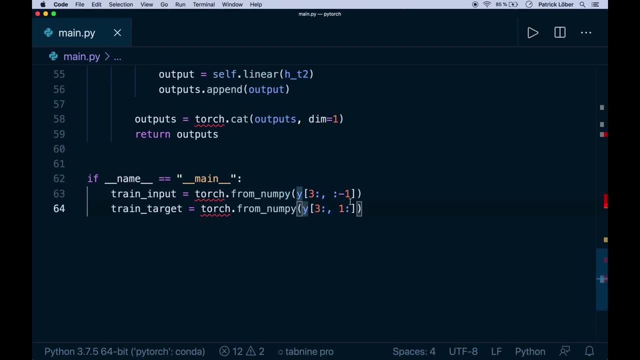 And then we have a y value We are going to quote and, after we already took this之前, sincronize 여기. that is shifted so that reaches one value more into the future, And with this we are then able to train our network. So we have the value of the previous position and then want to predict the 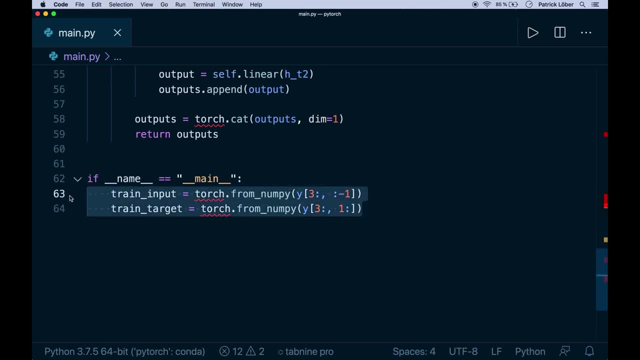 value of the next position. So this is what we do here. And then we also need test input and test targets. So test input and test target, And here again we want a shift that tends or. but now we only want to have the batch or the samples one, two and three. So we start at the beginning and go. 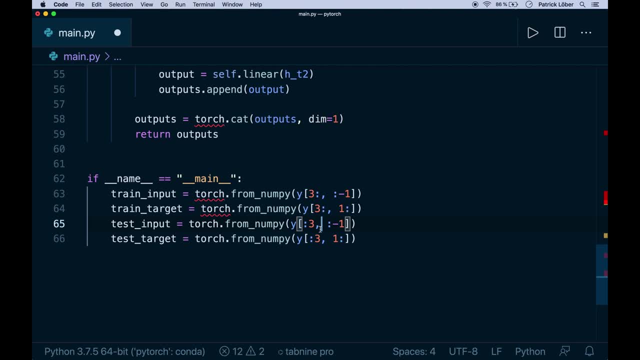 until three excluded. So this will give us the indices 1201 and two. So let's write down the actual shapes here to make this a little bit more clear. So our y has the shape 100 by 1000. And now this has the shape 9799999.. And this is the same 97. 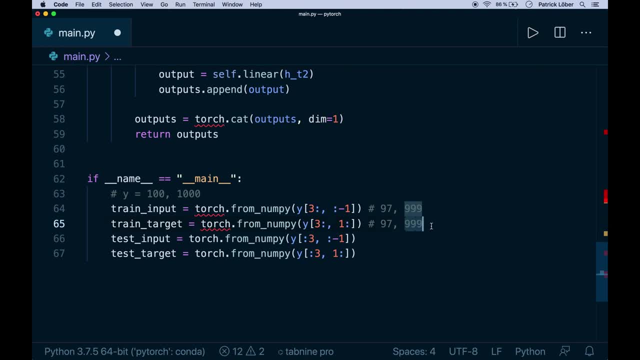 samples and 999 values for each sample- And here we only have three samples and again 999 values, and the same for the test targets. So now we have this and now we create our model with the Mix split, which will be our sample color, And this will give us the values, as now. we have this sample and now we created our multiple samples, But we also want to do some vouer plus, get to the point. we want to have this music And with this we have three samples And s, I guess, name this as our target target. And now we want to add: Yes, and I sketch the three has to 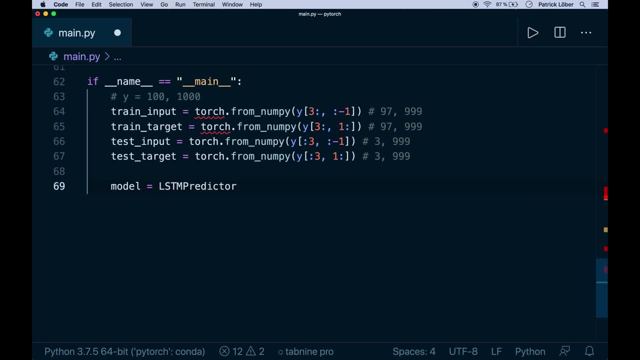 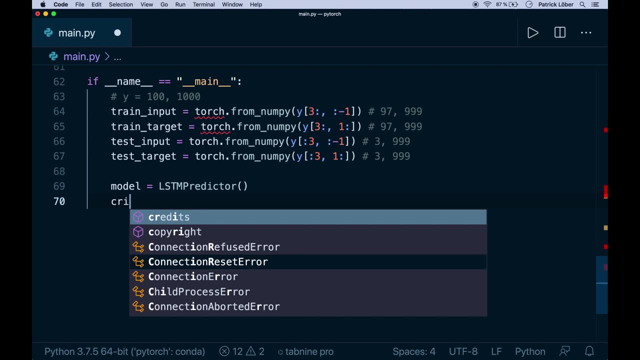 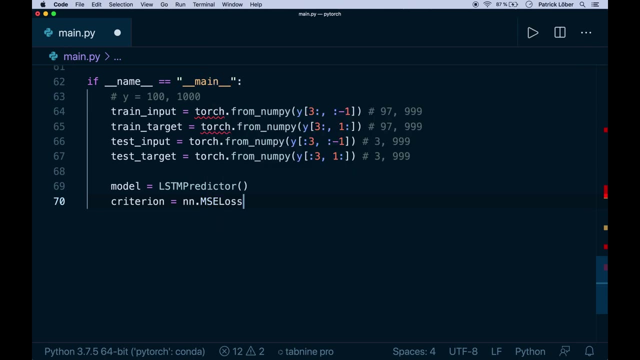 model. So our model equals our LSTM predictor and the hidden size. we leave this as 51.. And then we need a criterion, so a loss function, And in this case we just use the MSE loss, so the mean squared error. And then we also need a optimizer, So let's say optimizer equals. 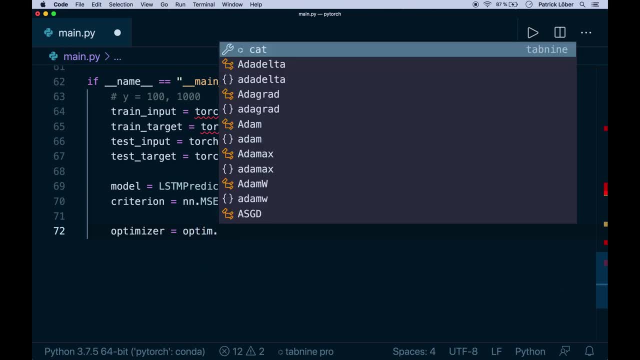 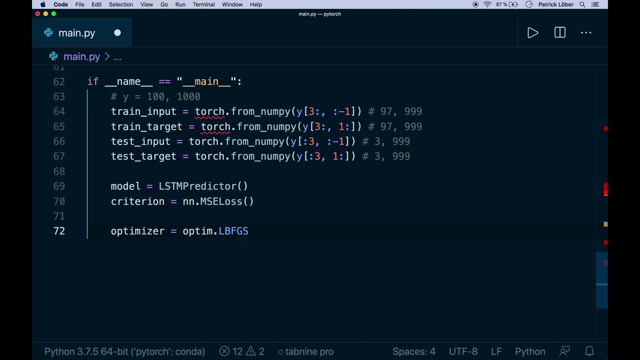 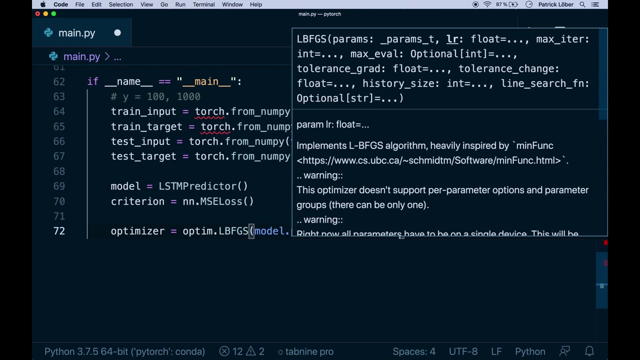 optim dots. And now here we don't use the Adam optimizer, So in this example I want to use the LB FGS optimizer And this needs the model dot parameters that we want to optimize And it also needs a learning rate. So model parameters and LR equals, and here I say point. 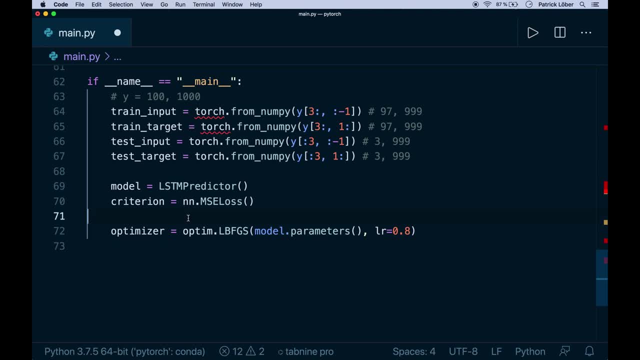 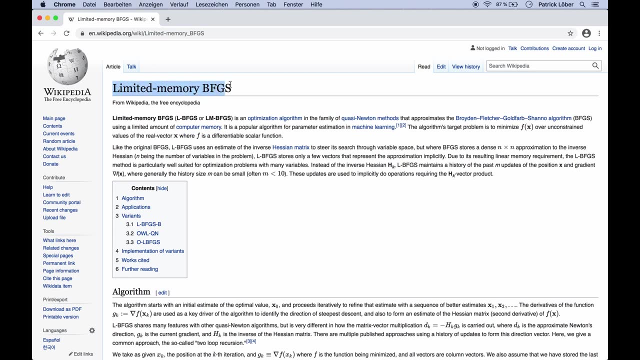 zero eight. So again you can play around with this. So I actually have the full name up here. So this is called limited memory B FGS And this stands for Broiden, Fletcher, Goldfarb, Shannon algorithm, And this works a little. 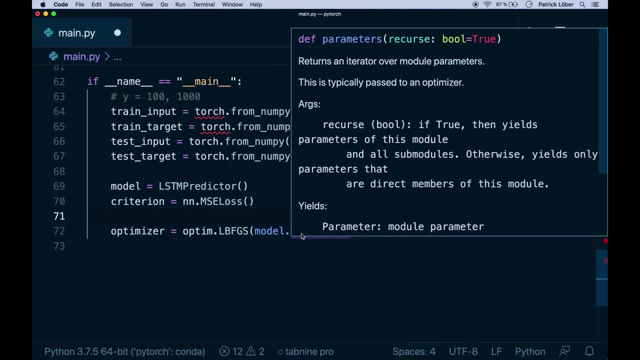 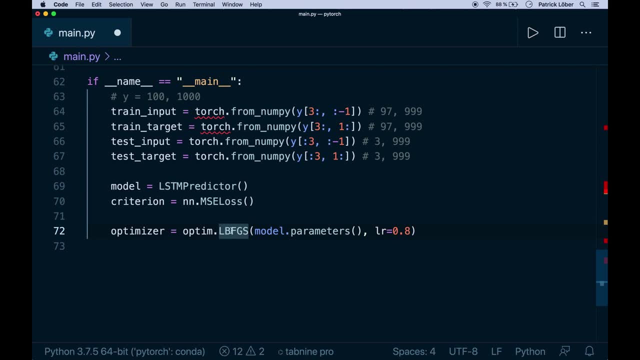 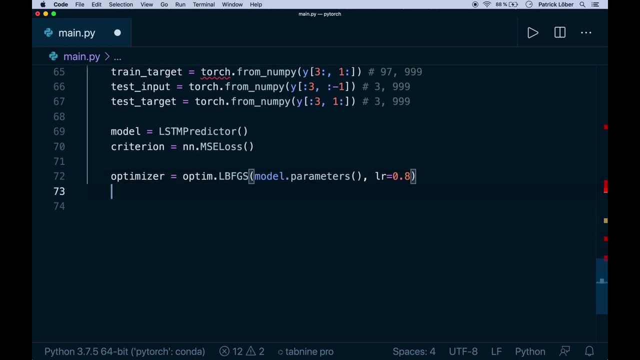 bit different than the Adam optimizer. So this optimizer can work on the whole data And it needs to have a closure, which means it needs a function as an input. So you will see how the this works in a second. So let's use this And then let's define the number of steps. 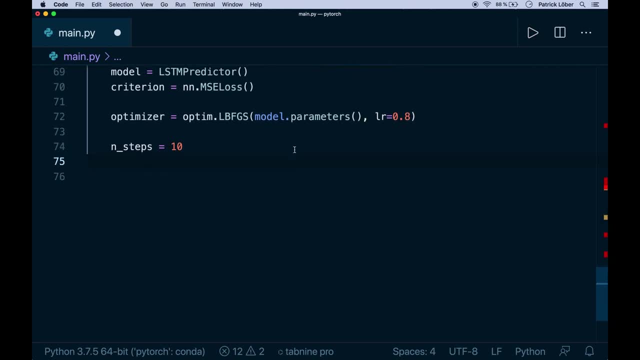 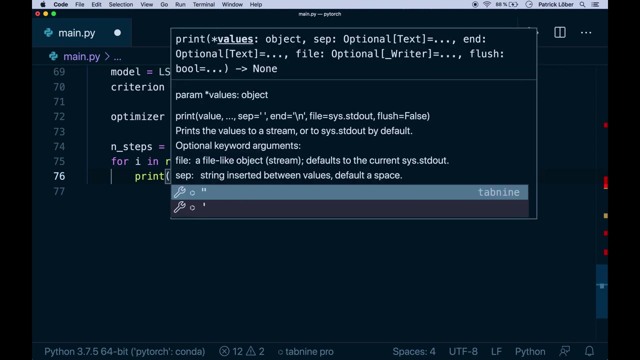 So in this example I only use 10 for the training in this video, So you can increase this a little bit to get an even better prediction, But for now that should be okay. So then I say for I in range, and then the number of steps, and first let's print the step step. 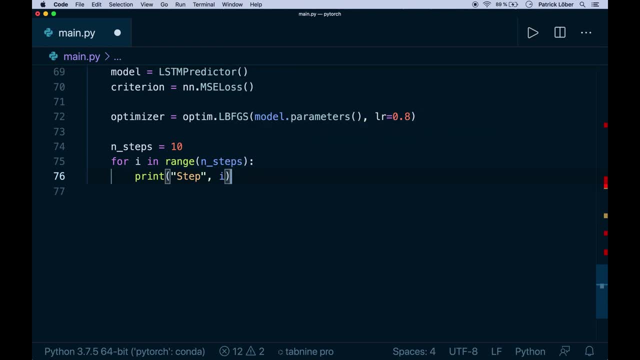 And then this is the current eye And then, as I said, we need a closure for this optimizer. So this, basically, is a function, So we define a function closure, and it don't has any made input parameters. And in here we need to empty the gradients, then we need to apply the loss, We need to 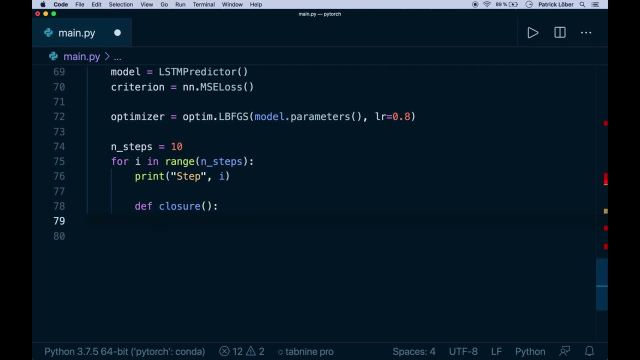 apply a forward step and then also a backward step and a Oh, our criterion. So here we say: optimizer dot, zero grad, then we call our model, So we say out equals model, and we use our training inputs here. then we calculate our loss by: 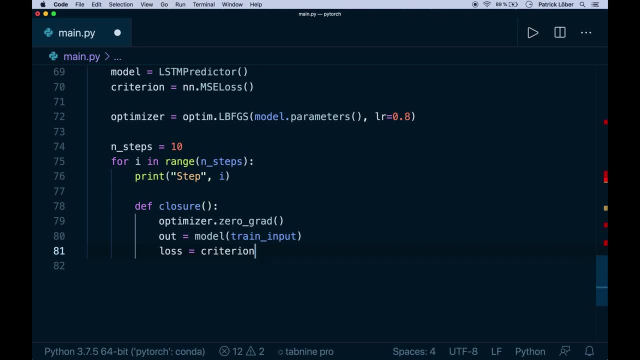 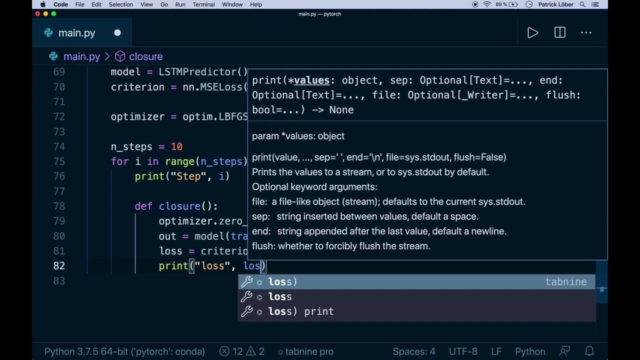 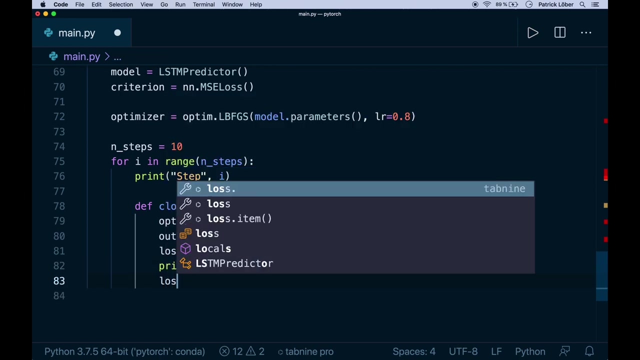 saying loss equals criterion, And here we put in out and our train target values, And then here we can say print loss, loss, And now he will say loss dot item, And after that we have have to say loss dot backwards to apply the back propagation, And then we want: 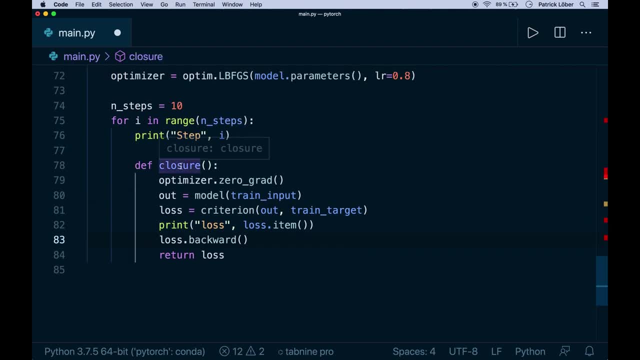 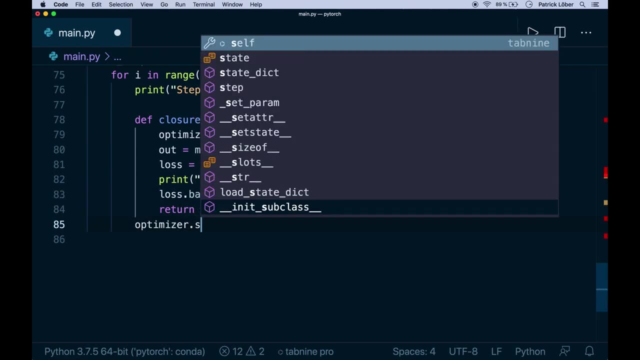 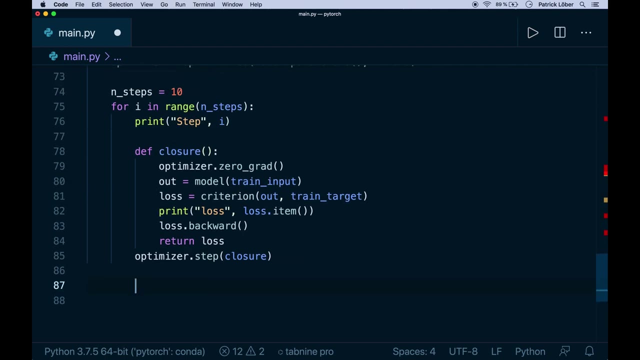 to return the loss. So this is our closure for the optimizer, And then after that we simply call optimizer dot, step And this needs the closure. And now we have this, and now we have a, have done the training in this step, And now we want to actually do the predictions, And for this 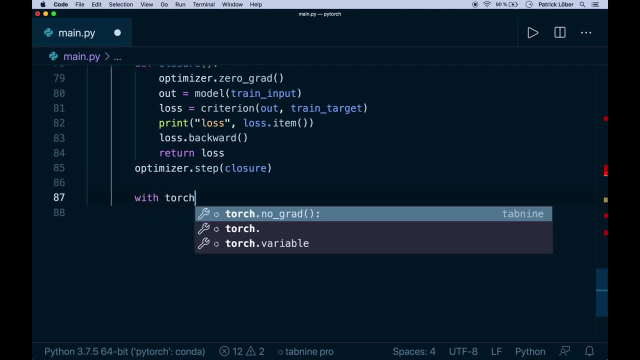 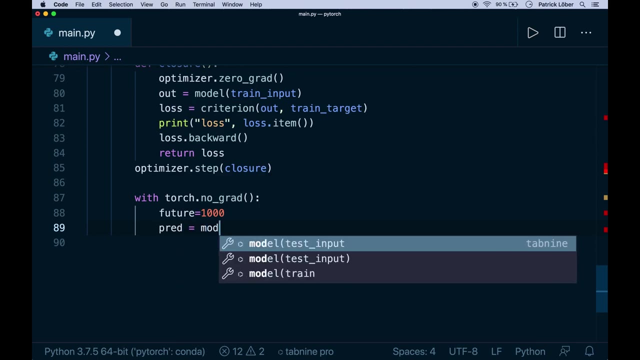 we don't need to track the gradients. So we say with torch dot no grad. and then we define the future values, let's say the next 1000 steps, And then we call the prediction, So pretz equals, and then again we call the model with: 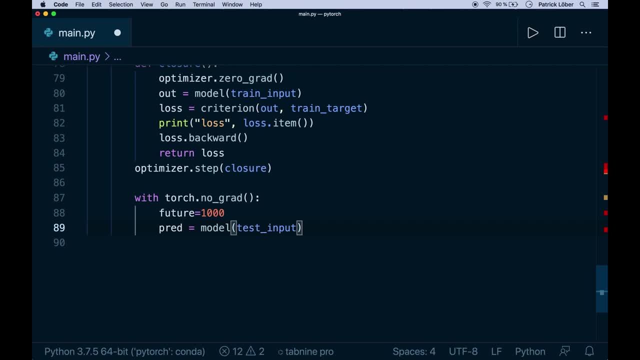 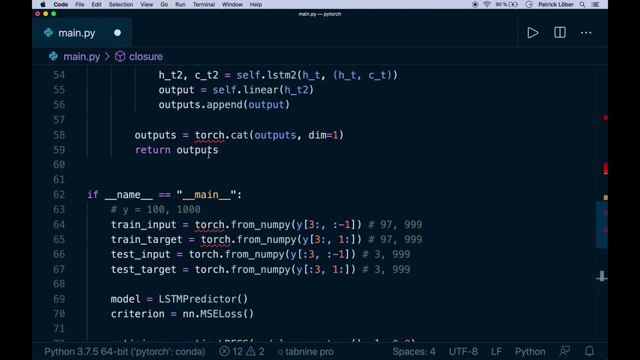 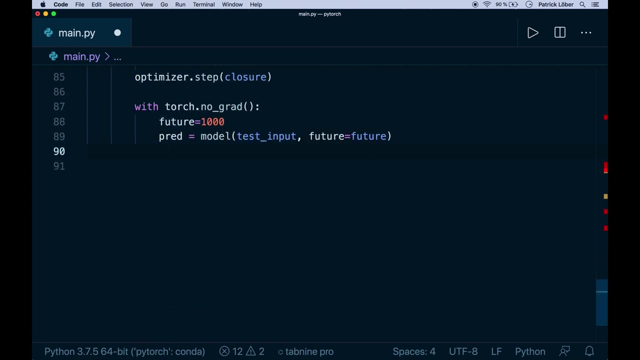 now our test input And, as the future future equals future, So this is the parameter that we can put in here. So now we actually do predictions with this, And then again we want to calculate the loss, So we say the loss. 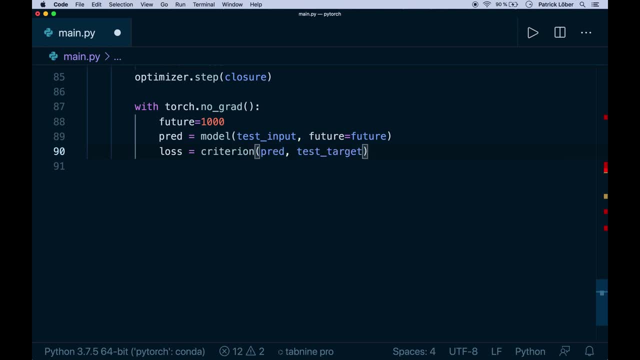 This is the criterion with the prediction and the test target. But now here we want to be careful what we use for the predictions, because for the test target we only have 999 values, But now our prediction also includes the future values, So we want to exclude them. 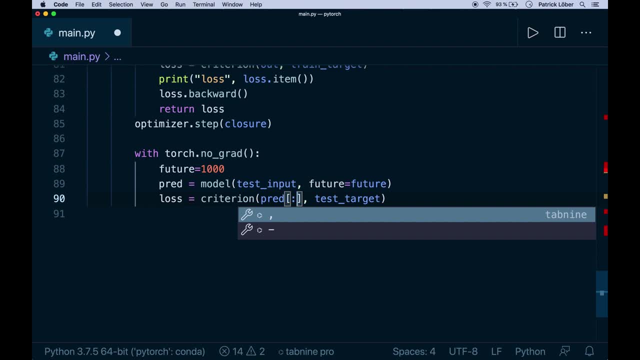 here actually. So here we use all the samples, so just a colon, And then we start at the beginning and exclude the last future values, So we can say minus future, like this, And then we print the loss. So here we say again: print, and this is our. 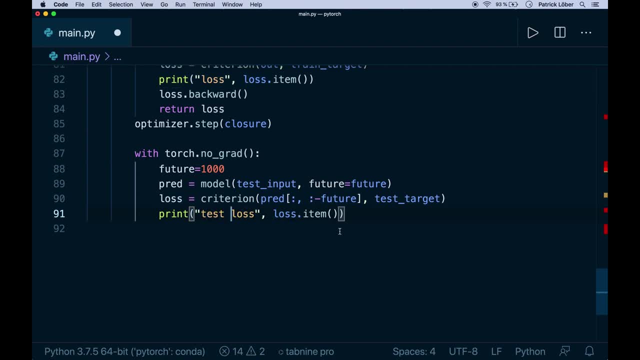 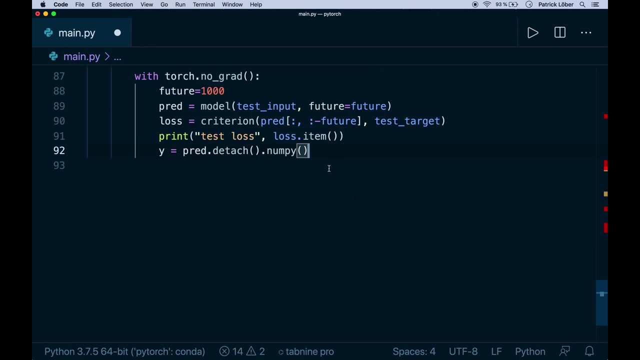 test loss, And then we say loss, dot item, And now we generate our actual y and use this as numpy array. So here we say: y equals prediction, dot, D touch, and then dot, numpy, And now we have this as numpy array and can use this for plotting. And now we want to plot this, And for this I actually 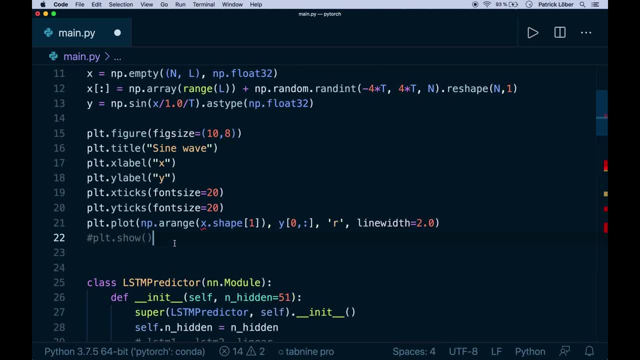 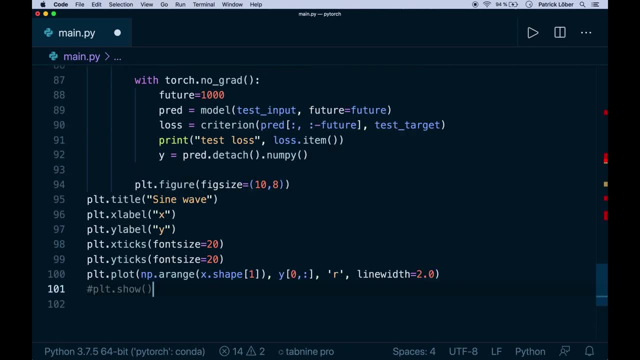 want to plot this into a PDF file So I can grab the code from here and then put it down here again as well And do the correct indentation, And we don't need this. And let's also change the fixed size a little bit, So this should. 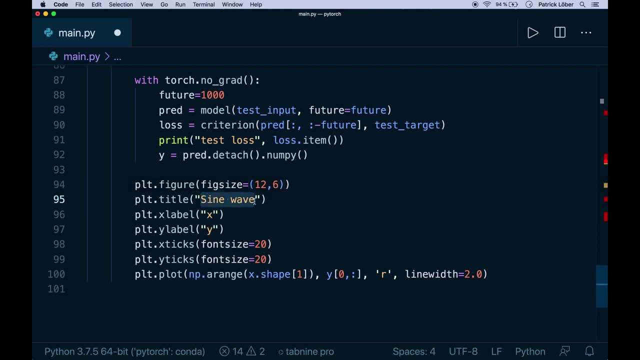 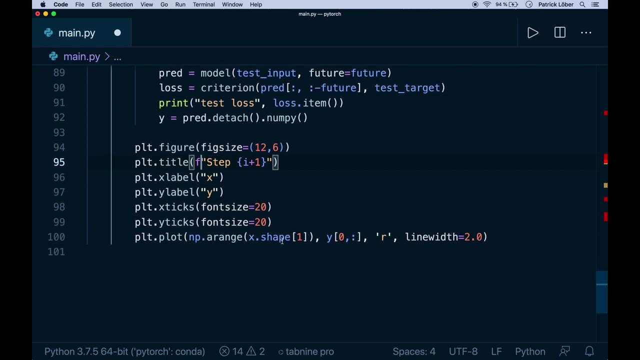 be 12 by six, And as the title here we say step, And then our step is: let's say: this is i plus one, and then it must be an F string And we can leave the rest as it is, And then we create a little helper function. So for this we say: you can use the pointer to do this. 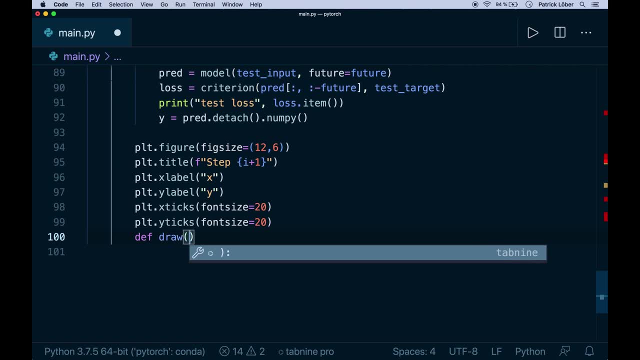 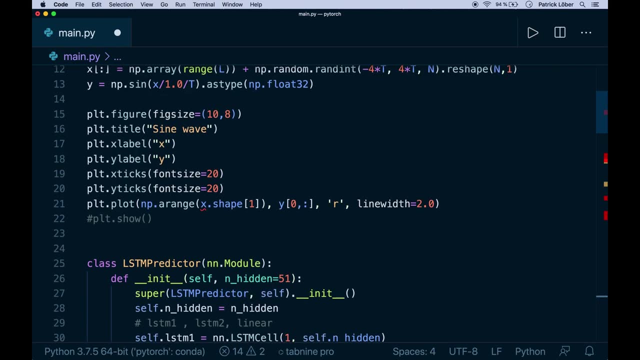 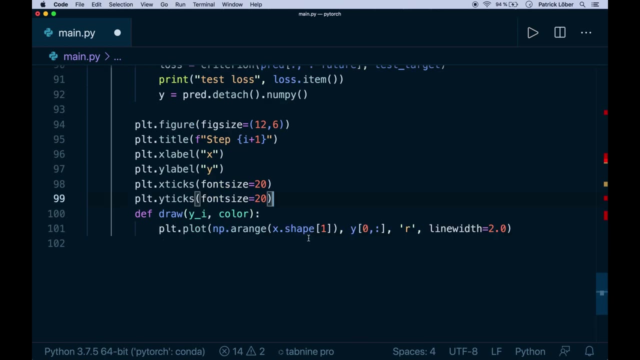 say define, draw. And then here we want to draw the current y, i, And we also give it a color. And then we grab the same command as we are doing here with the arrange function. And now for the shape: let's use n equals, and this is: let's use train input dot shape. 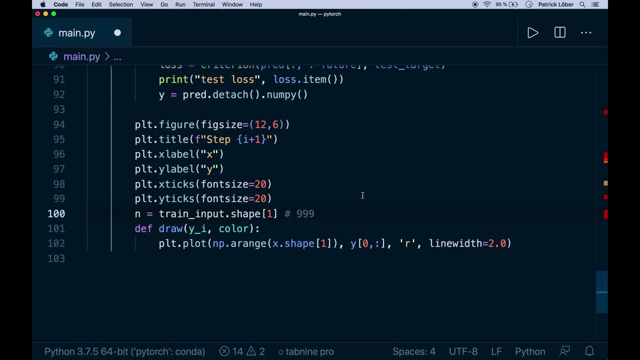 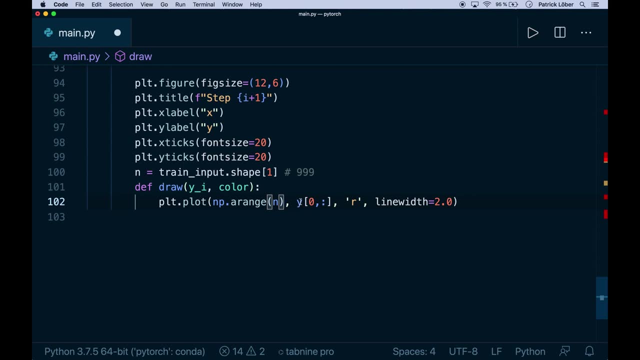 one. So this should be 999 values. So here we put in n. So this is what we need at the x axis And at the y axis we want to have y, i and starting at the beginning until n. So the first n values from zero to 99999.. And this is our color parameter. So these 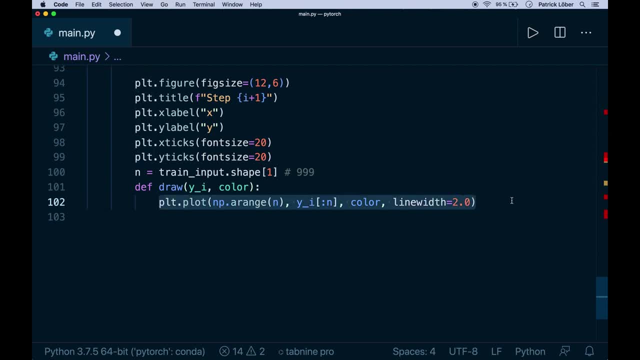 are our actual values That we have. And now we want to predict, to plot the predictions. So here we want to say: arrange from 999 until n plus future, so until so the next 1000 values. and here we start at n and go until the end. So n, colon, the end. 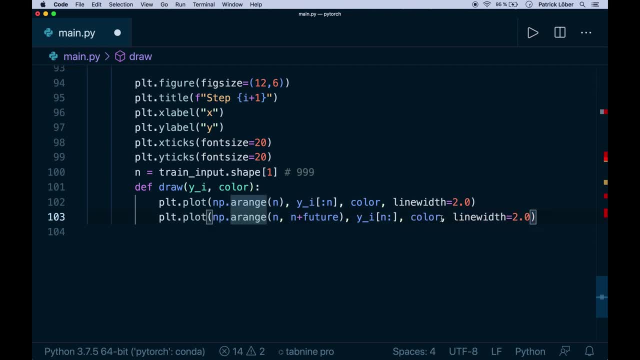 So these are the values that we need. So, and now we want to plot the predictions. So are our predictions. So let's call them, let's plot them in a slightly different style. So we say color plus and then colon, So this will put it in a dashed style. So now we have 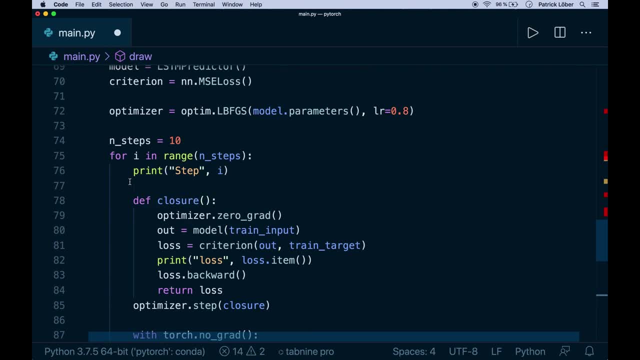 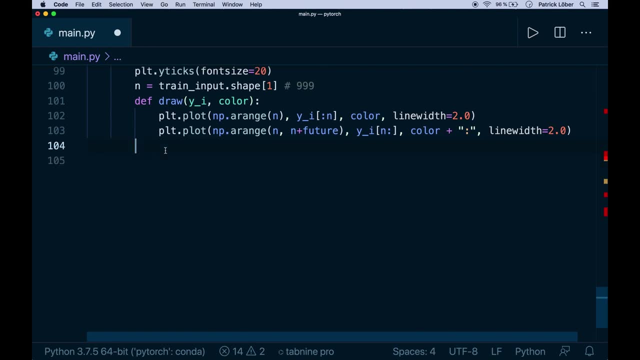 this helper function And now we draw the first three test samples. So we only have three test samples, So we plot all three of them. So for this we say draw, and then let's say y zero, And as a color let's use red. then we again do this for y one and y two. 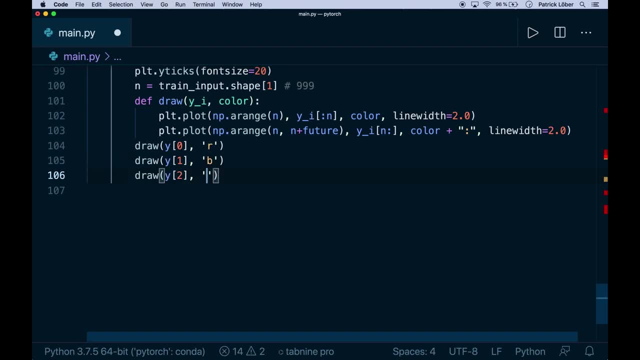 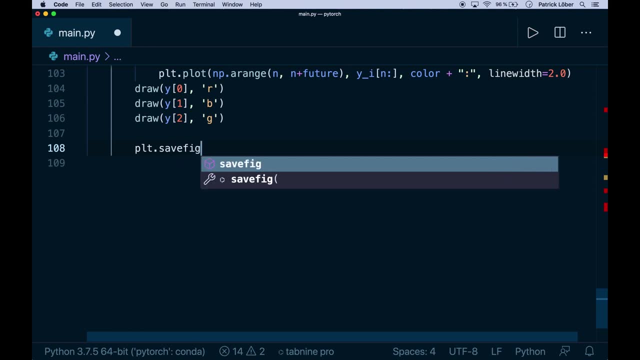 And let's hear you use blue and green for the colors. And then after this we want to say PLT, dot, save figure. And now we can save this in a PDF file by simply saying predicts. And then here let's use percent d, dot, p, d, f, And the parameter percent d is just our current step. And then 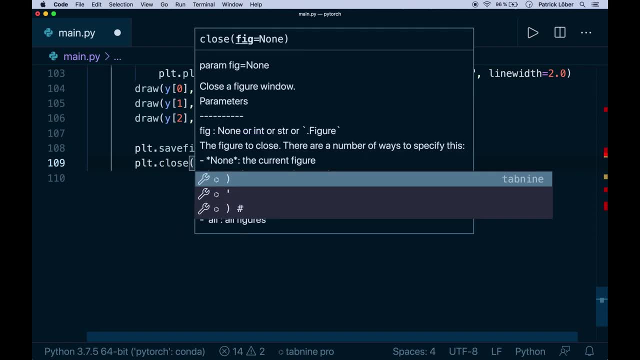 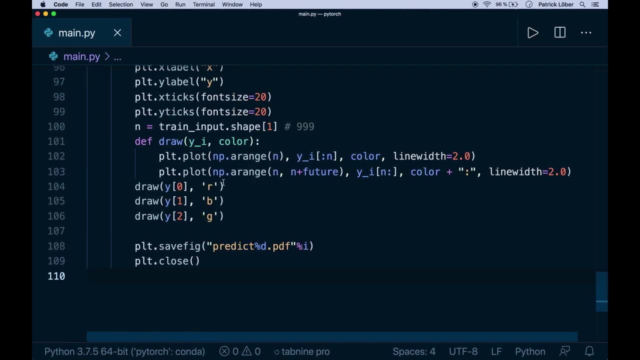 we have to be careful and have also have to call PLT dot close to close the file. So now this is everything we need, So let's run this and hope this will help us. Alright, so now we can see that everything works. So let's clear this out and say Python. 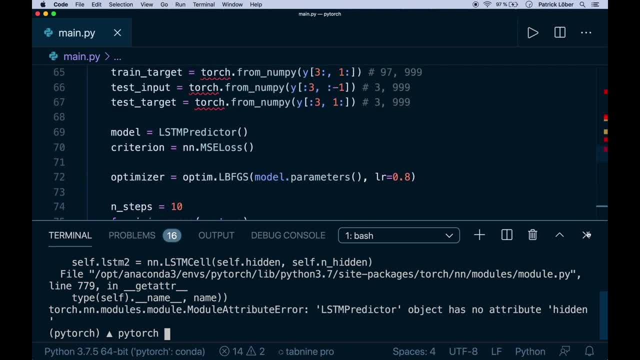 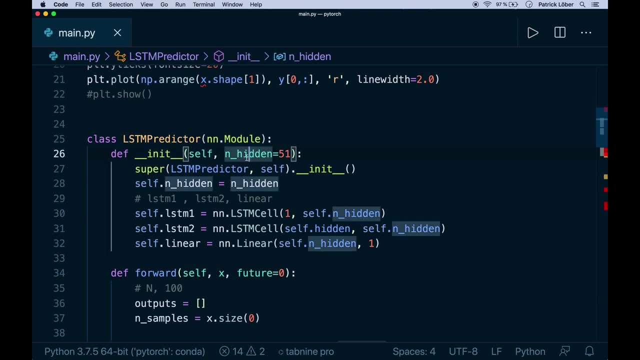 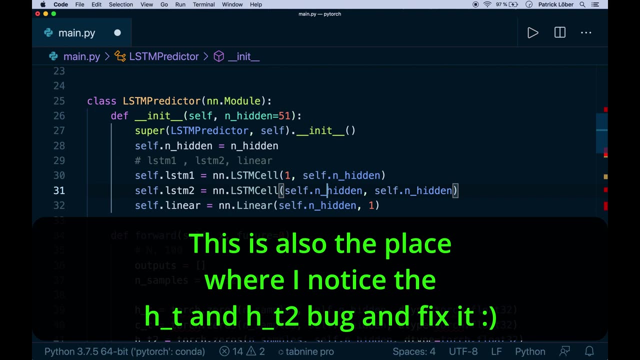 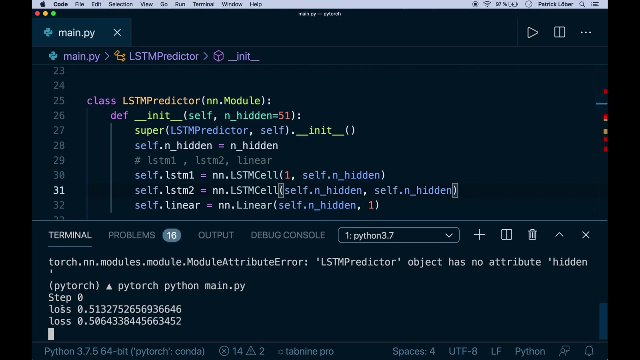 main dot pi, And I think I have a typo somewhere with an hidden. So let's have a quick look- and hidden. So we do have this here And we also have this here, And here I have the N missing So and hidden. So let's test this again. Alright, so now we can see the log. 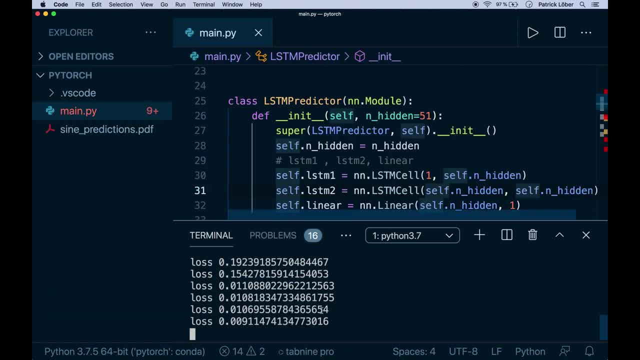 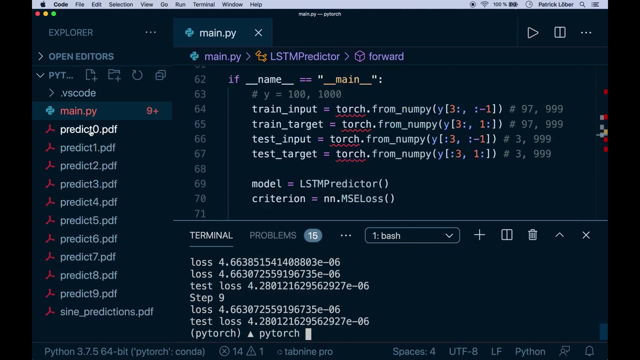 being printed in here And now. if we monitor our folder, then you might see the PDFs appearing here. So let's wait until this is completed. All right now. so training is done And we can see that we have 10 new PDF files here. 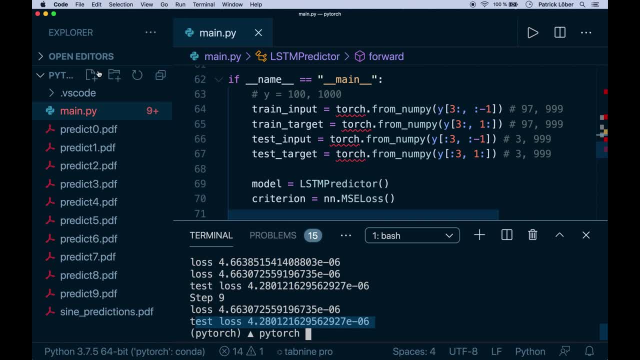 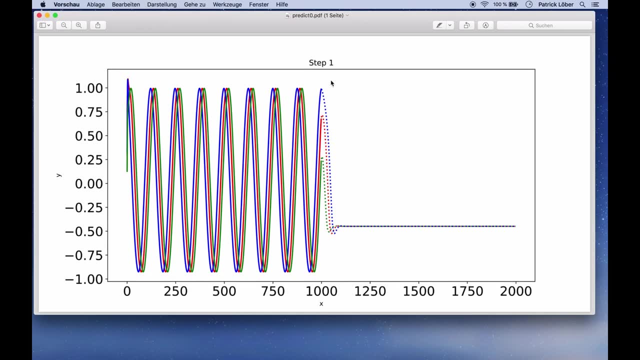 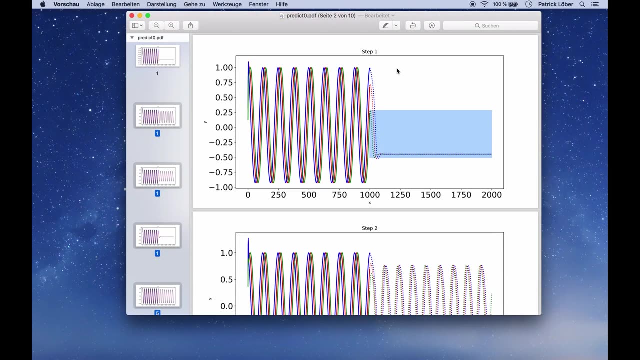 And we also see our final test loss. So this is pretty low. So I hope that we can see accurate predictions. So let's have a look at those PDF files and let me actually put them into one file for you, All right? so after the first step, we can see that our predictions are not very good.